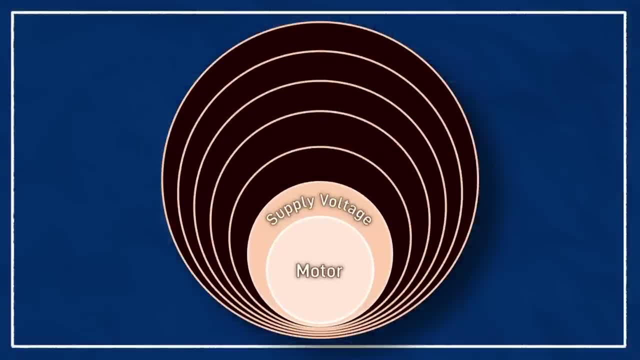 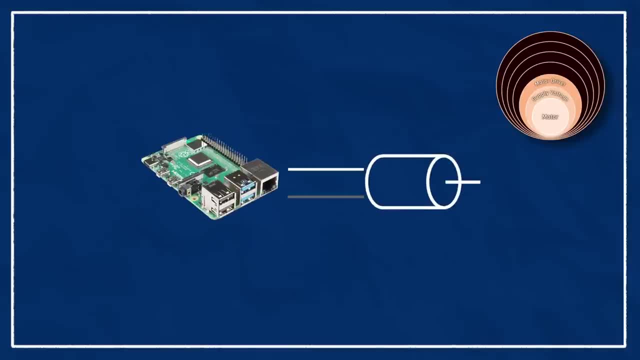 and no way to control it remotely. So the next layer that we're going to add is a motor driver. Part of the reason we can't just plug a motor straight into a Pi or an Arduino is that motors require a relatively high voltage and high current compared to what the pins on these chips can handle Instead, 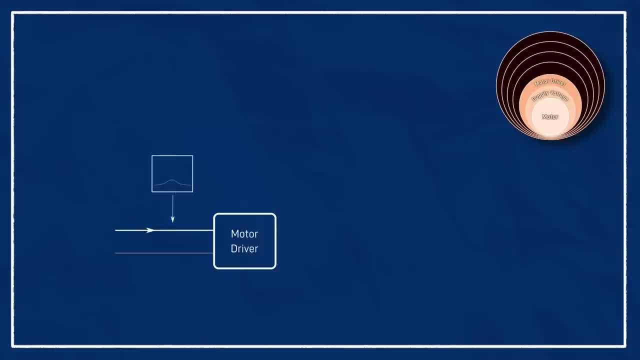 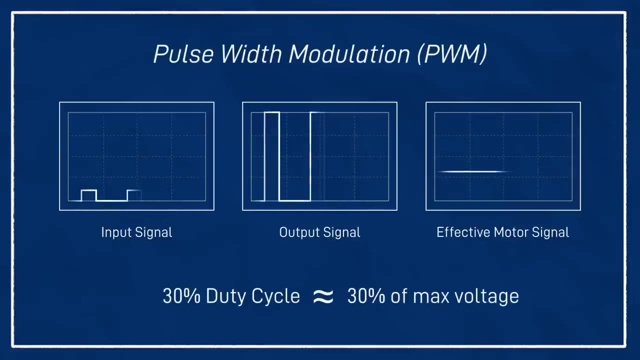 we use a motor driver. This little board takes a low voltage, low current signal from some kind of controller and uses our power supply to amplify it, creating a higher voltage, higher current feed to drive the motors. This signal is usually PWM, a series of fast pulses that, when you average them out over 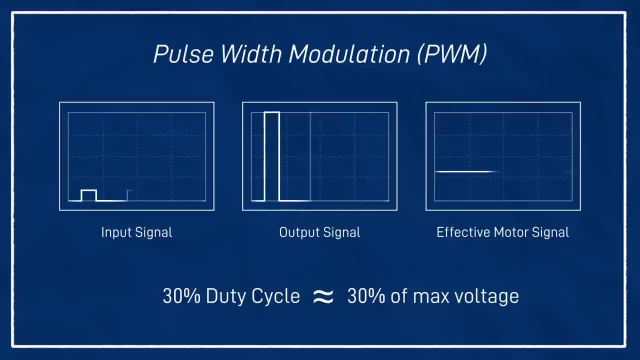 time. the ratio of on time to off time, called the duty cycle, determines the percentage of the total voltage that a motor effectively sees. Basically, the shorter the pulse is, the slower the motor will go. the longer the pulse is, the faster the motor will go, and if the pulse is on 100% of the time, then the motor's going. 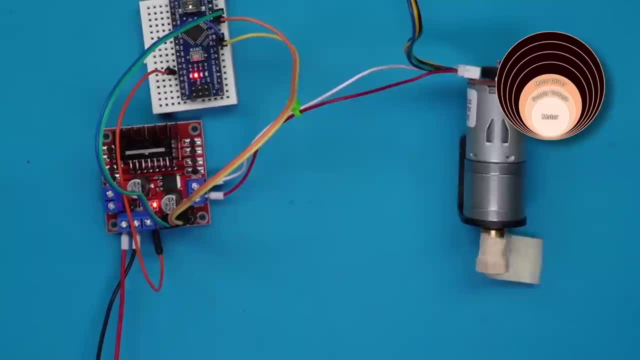 to be going full speed. So here's that motor from before. I've got it hooked up to a motor driver with some other circuitry off screen and I can make it go fast or slow or even backwards. So that's our motor driver. but now we need a way to generate that PWM input signal and 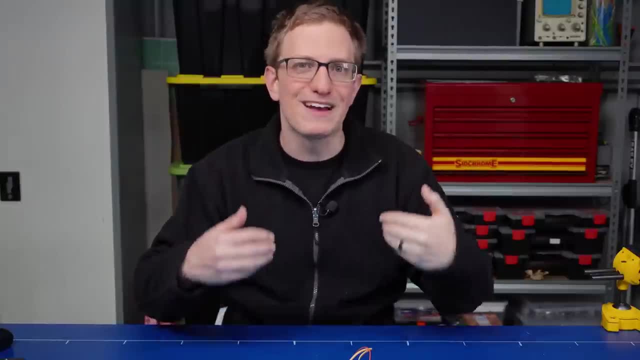 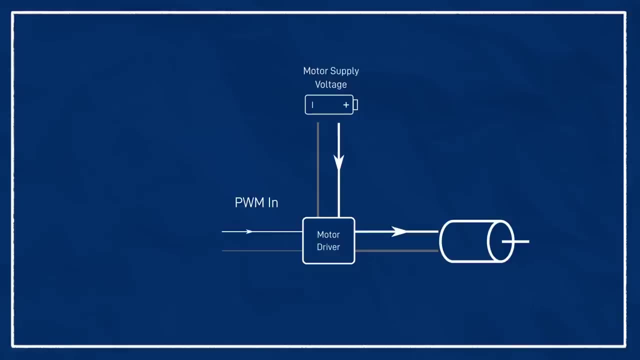 for that we'll use a motor controller. Now let's just pause for a second and talk about terminology. It's a bit vague, but the way I use it, a motor driver is a circuit that just blindly takes an input signal and amplifies it to send to the motor, Whereas a motor controller is a bit smarter because 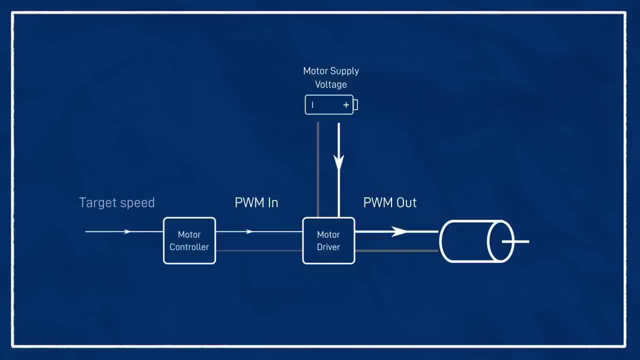 it's input is in a more practical format, maybe a target speed or a target position, and then it calculates the appropriate signal to send to the driver to get the motor to go the right speed. Sometimes both of these will be combined into one circuit. especially you'll find this with 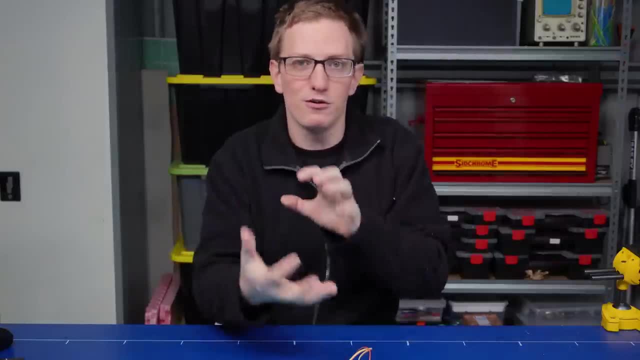 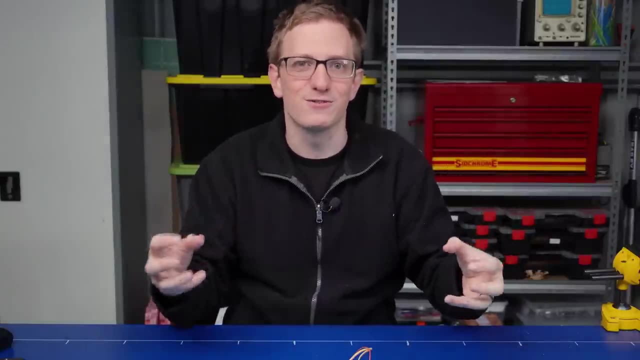 brushless motors because they're a bit more complex, or sometimes they'll even be all bound up in one unit with the motor itself, like with a servo or a dynamixel. Conceptually, though, we're going to keep the driver and the controller separated. 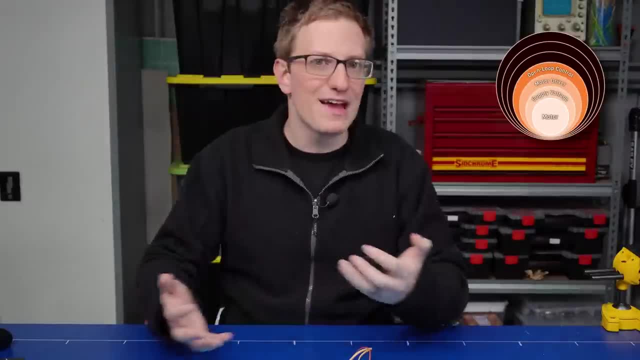 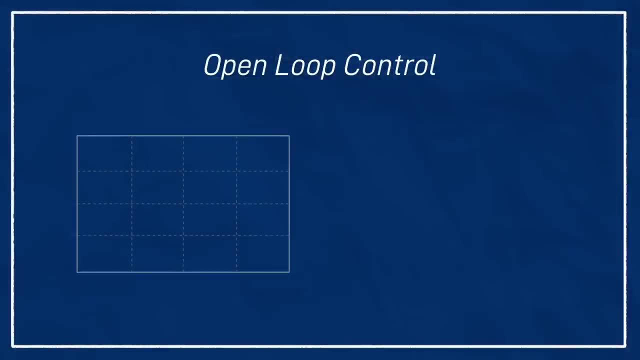 The simplest kind of motor controller is an open loop controller. This is where we have some kind of predefined map between our input signal and our output signal. If the robot is ultimately being driven by a human, this can be as simple as taking the operator's joystick signals and mapping 0% to 0% and 100% to 100%. but if we want 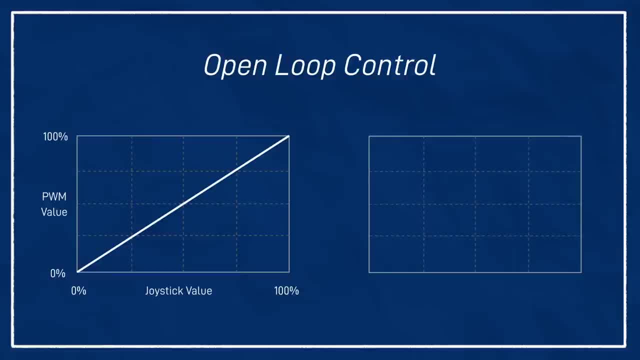 to start getting a bit more automated. we can try to come up with a function that maps our requested input speed in whatever unit- maybe degrees per second- to the appropriate PWM value, And we can figure out what this function is by testing a bunch of input values. 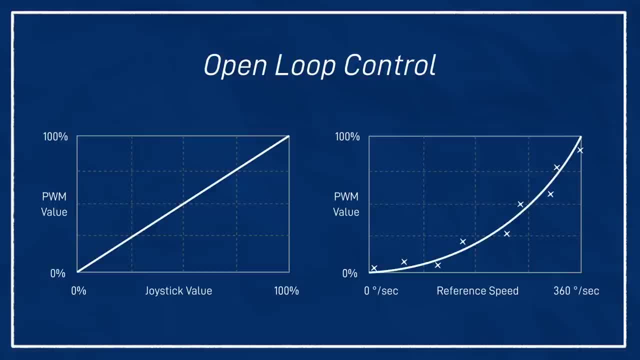 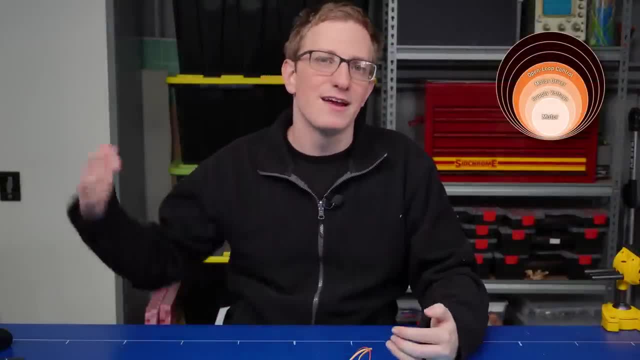 measuring the speed we get out and fitting an equation to the input value. So let's go ahead and do that. Although this approach is really simple and it might be good enough for some applications, it tends to fall down pretty quickly. The appropriate speed to driver signal function. 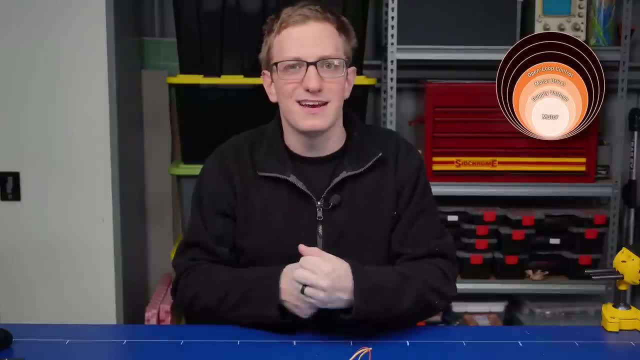 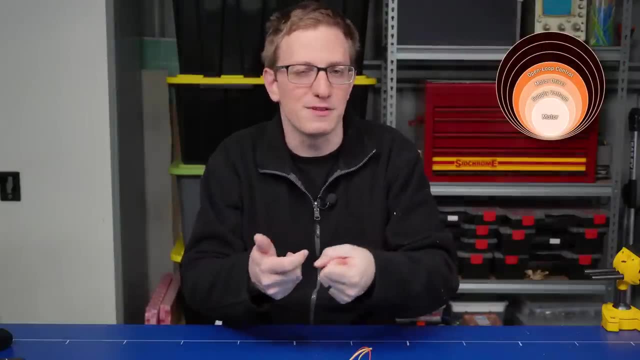 can change depending on a whole lot of factors: The load that the robot's under, the battery charge, or even if the motor is going forwards versus backwards. A human operator can naturally compensate for these with slight changes, but if we want to do robust automation, we 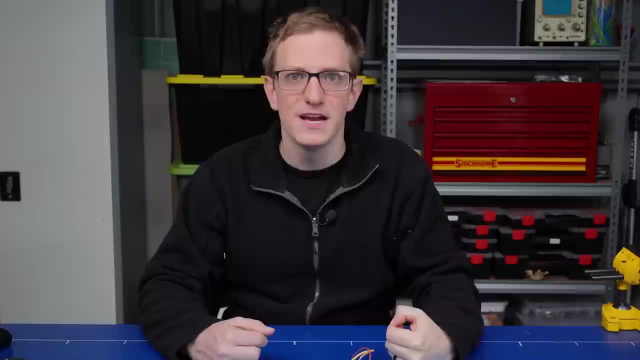 really need to be able to command our motors to go an exact speed. To achieve this, we need a way to measure the speed of the robot. We need to measure the actual speed of the motor live and feed that back into our controller. 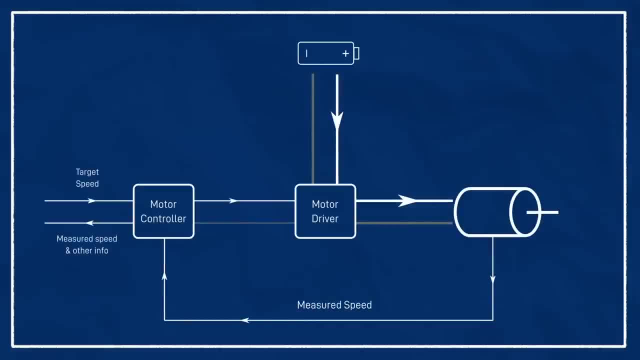 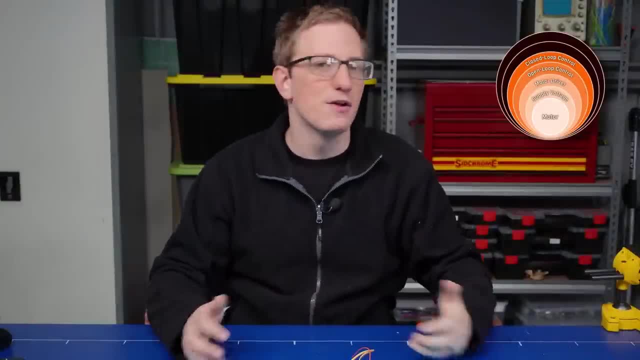 so that we can adjust our input until we're getting the speed exactly right, And this is called closed loop control or sometimes feedback control. There are different kinds of closed loop control methodologies. We're not going to go into them now. The most popular one is called PID control. I'll try and find a video and include. 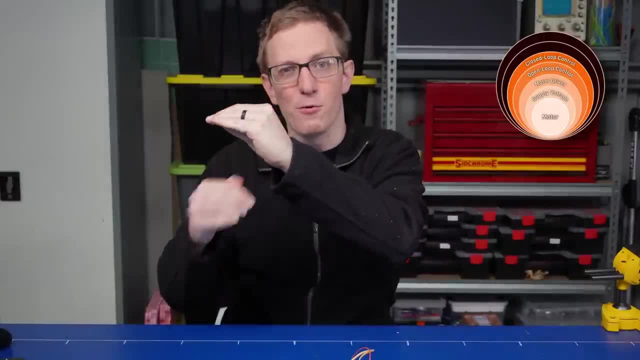 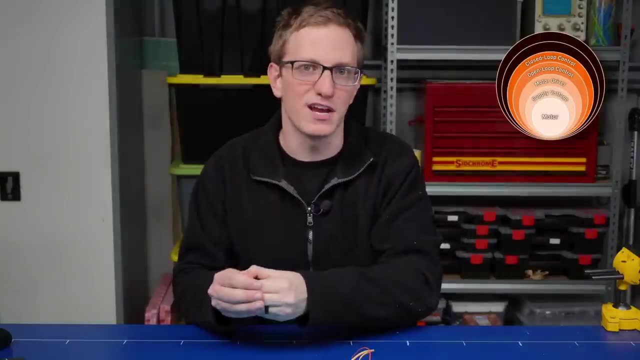 a link to it. But basically we look at how far we are away from where we want to be and adjust our signal accordingly. So if we're really far away, we make big changes and if we're not very far away, we make small changes. 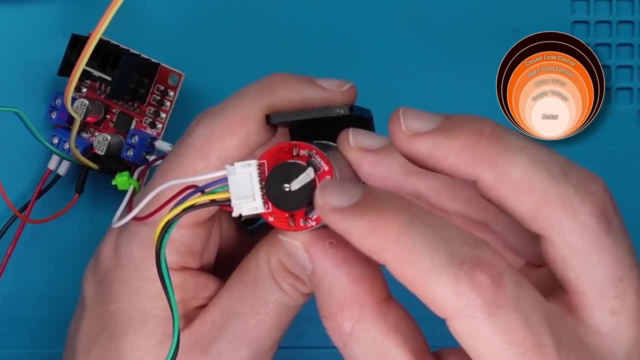 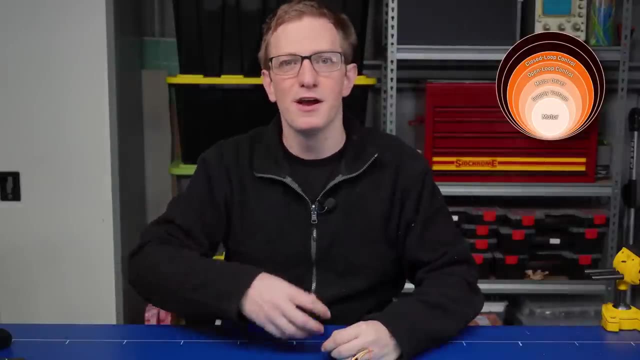 And that's why the motors I've got have encoders on them. As this little wheel on the back of the motor spins around, it'll send a signal back to the controller that we can use to calculate the speed. So, whether it's open loop or closed loop, off the shelf or custom built, like we'll see, 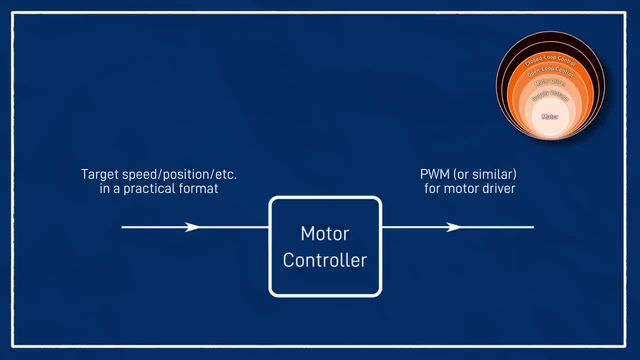 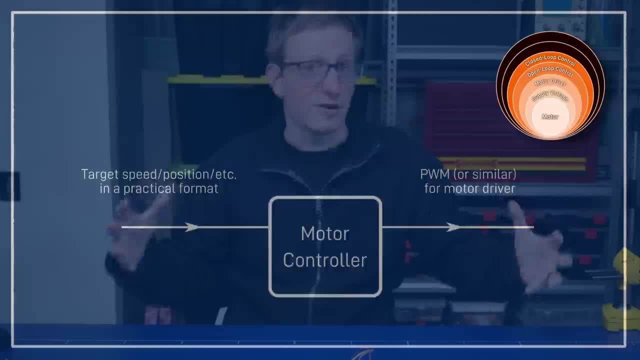 in a minute. our motor controller is able to take a target speed or sometimes a target position in a format that's good for us, and it converts it into a signal for that driver And that way our robot controller, in my case the Raspberry Pi, is able to just send. 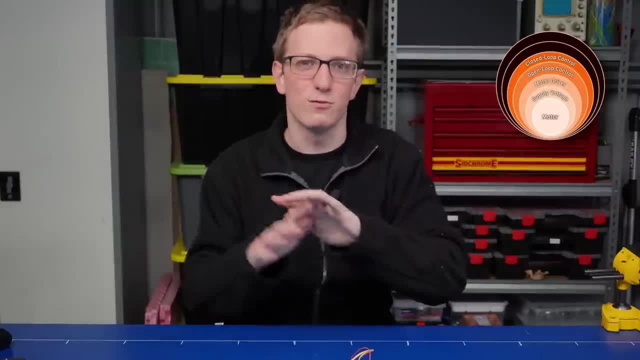 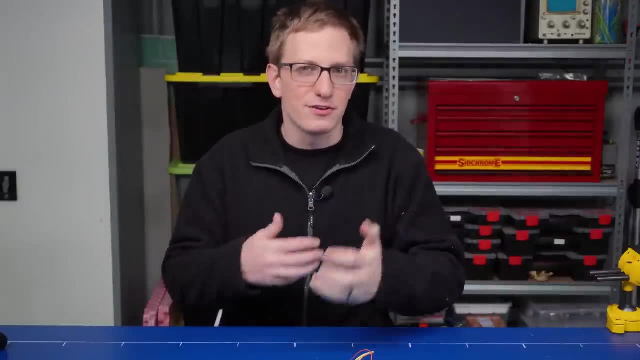 the speed that it wants and the motor will go that speed, and it doesn't have to worry about all the low level details. The motor controller takes care of that. Now you might be wondering: can't I just implement that kind of control straight on the Raspberry? 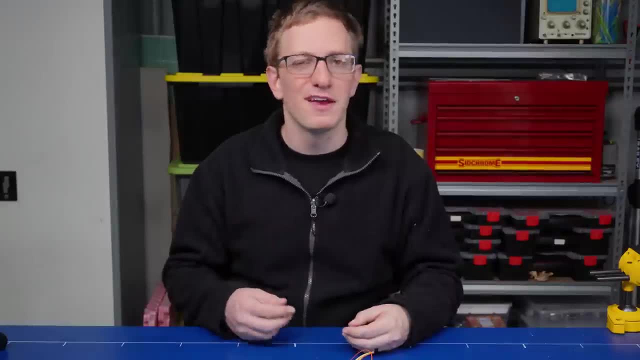 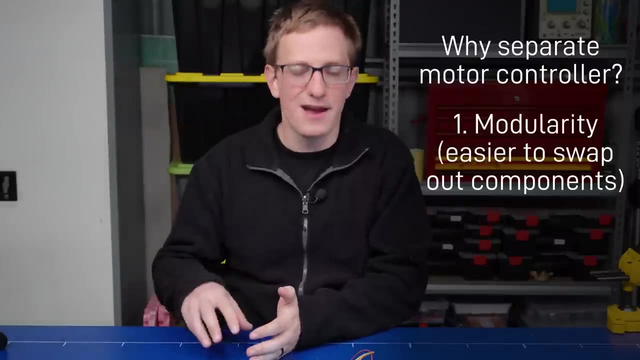 Pi itself, And you can, but I don't necessarily think you should. There are two main reasons for that. Firstly, it keeps the system more modular. So imagine, later on down the track, you instead wanted to swap out your motors for something that has its own controller. 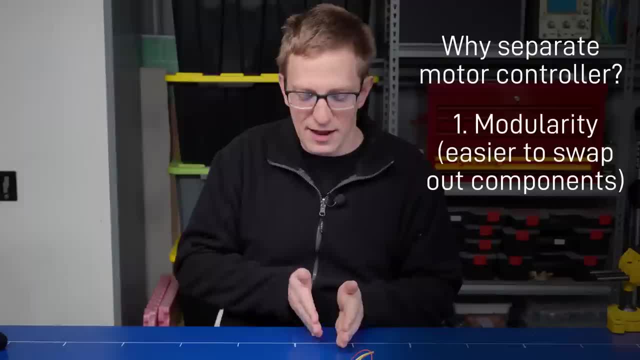 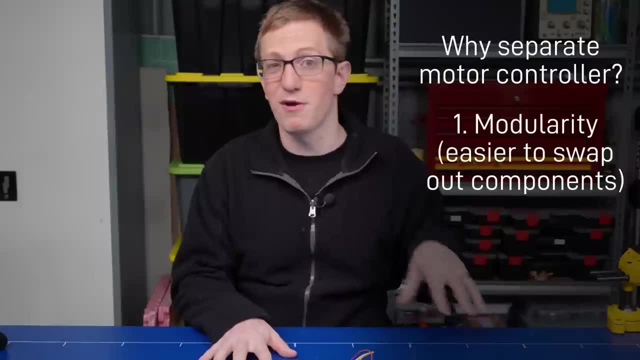 maybe like a Dynamixel. Having done it this way lets us create a kind of a divide between two parts and we can more easily separate that component, switch it out. Maybe you want to switch out the Raspberry Pi itself for a different board and keep our motor controller. 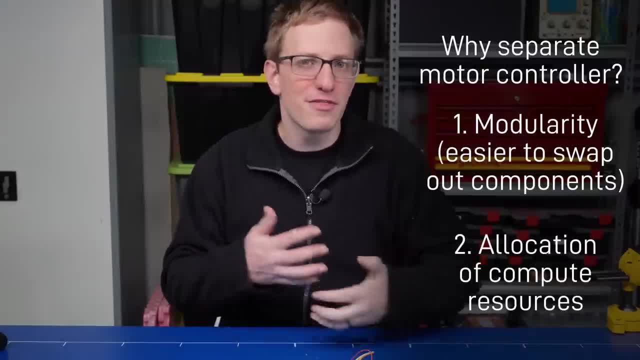 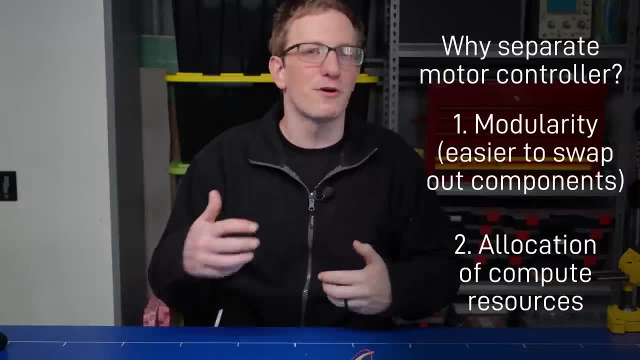 the same. Secondly, it means you never have to worry about other things on the Pi interrupting the control system code. You can imagine that maybe the camera code decides that it wants to hog the processor and all of a sudden your PID loop is taking 10 seconds to process. 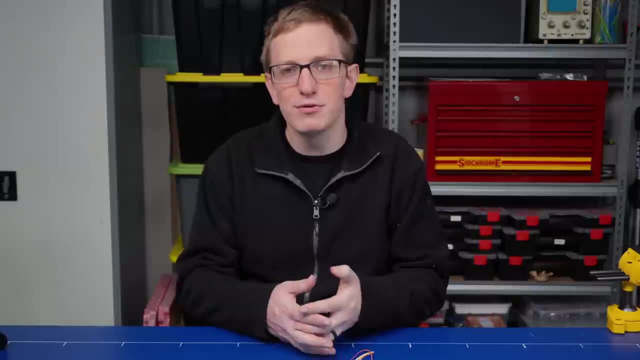 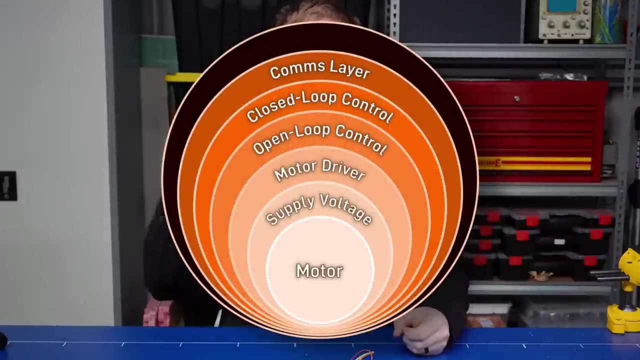 and your motor's off doing something weird. If your motor controller is on the same board as your robot controller, maybe in a simpler robot it does make things easier, But otherwise we're going to need a way to communicate. We need some way for our main. 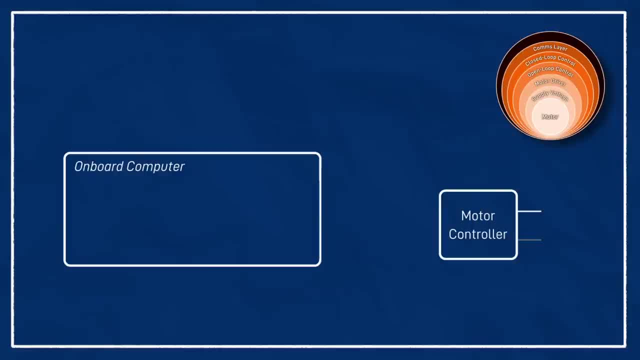 robot controller- the Raspberry Pi in my case- to transmit speed requests to the motor controller and then a way for the motor controller to potentially feed information back, maybe speeds or positions, or even currents or temperatures. It'll vary depending on the controller, but 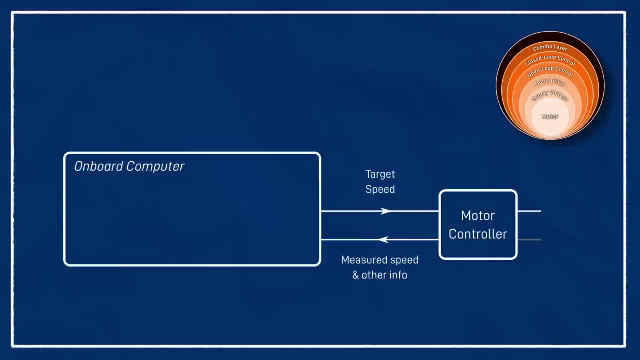 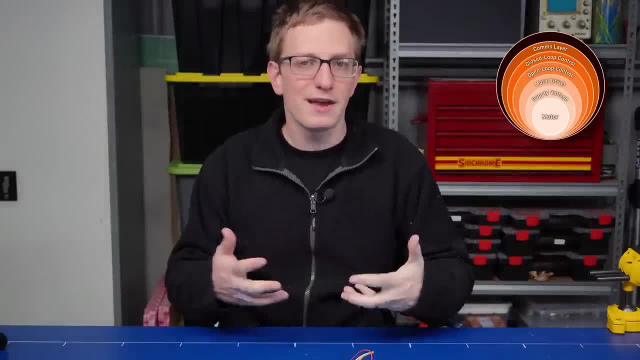 these comms will often be some kind of serial line, maybe RS232,, 422,, 485, or sometimes something else like CAN, I2C, even PWM. In my case, I've got a Pi communicating to an Arduino using serial over USB. 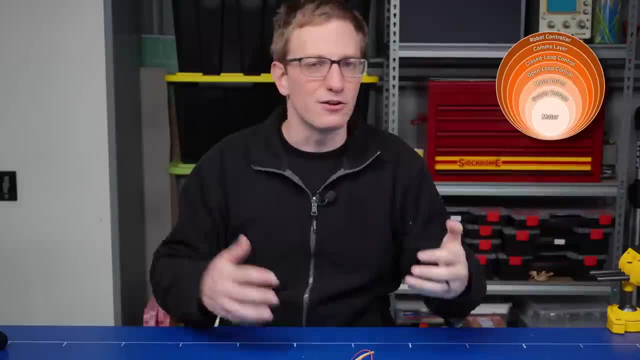 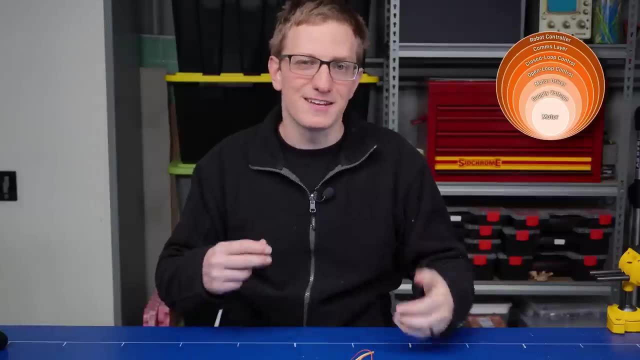 So the final stage is the overall control software for the robot And on any reasonably complex robot, this is going to be running on some kind of onboard computer like a Raspberry Pi. This software is going to need to do two different things. Firstly, it's going to need to calculate. 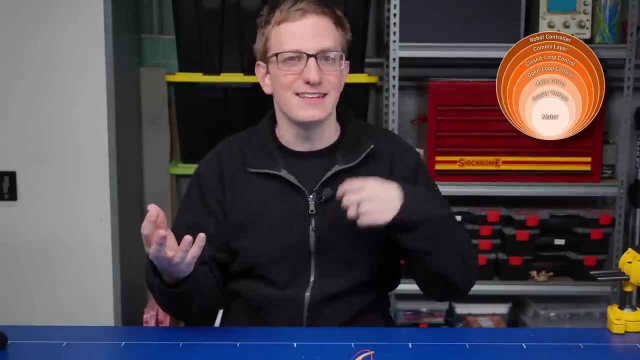 the speeds that it wants the motors to go for its application. And then, secondly, it's got to transmit those speeds, using the appropriate protocol, to the motor controller. So I'm going to split these up into two parts. The first part is going to be the motor controller. The second part is going to be the controller. So I'm going to split these up into two parts. The first part is going to be the controller. The second part is going to be the motor controller. The third part is going to be the controller. The fourth part is going to be the controller. 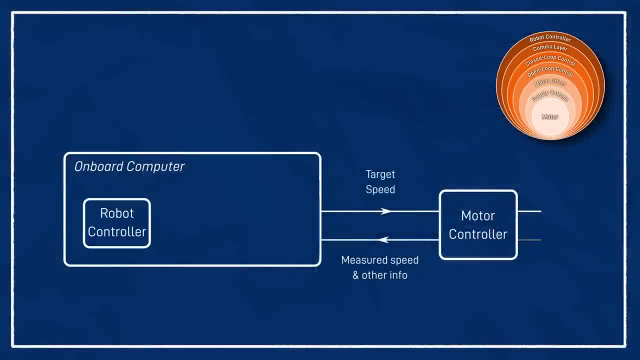 So I'm going to split these up into two separate conceptual components. I'm going to call them the robot controller and the driver software. not to be confused with the motor driver. This could look a little bit different depending on your exact setup. So maybe all of the code. 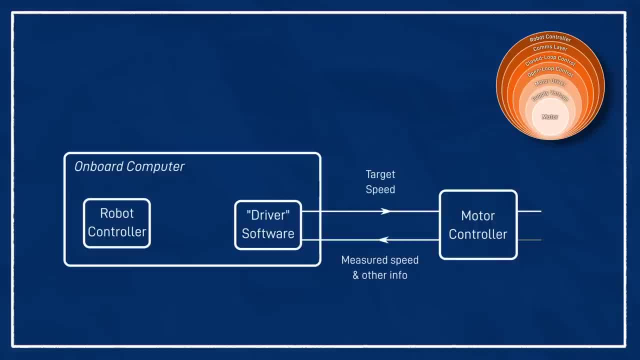 is in one program, but the driver is a separate library that it loads. Or if you're using regular ROS, then maybe these are two different nodes that are communicating using topics. Or if you're using ROS2 control, then the controller will be a ROS2 controller and 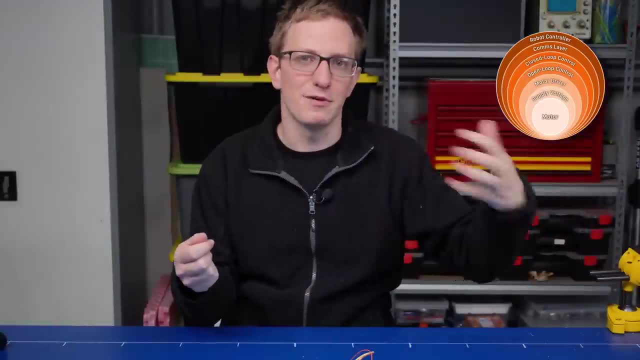 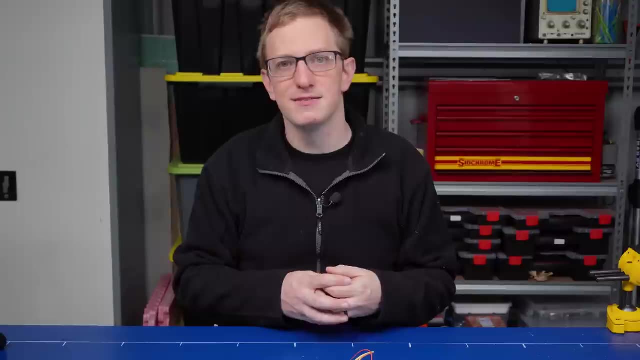 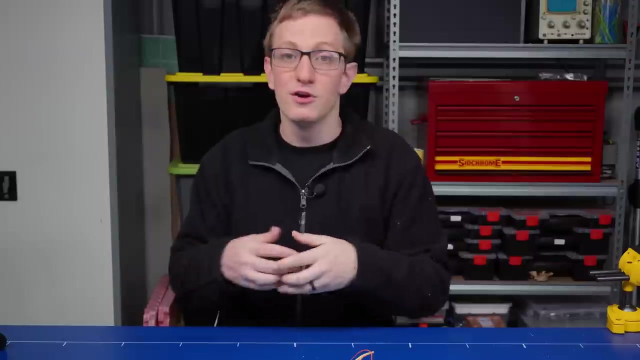 the driver will be what they call a hardware interface. So this is the rough structure that we use pretty much whenever we're going to be using motors in robotics. Realistically, it's not going to look the same for every situation. Sometimes you might have the motor driver and the motor controller on one board, or 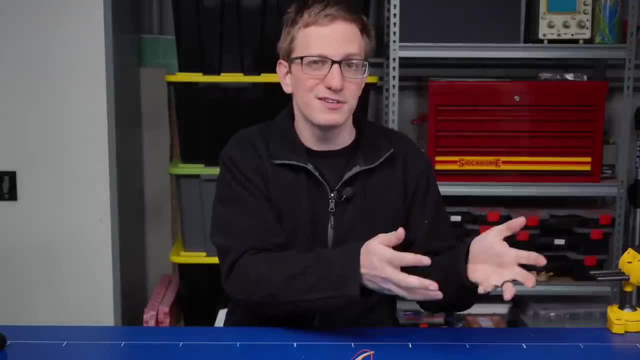 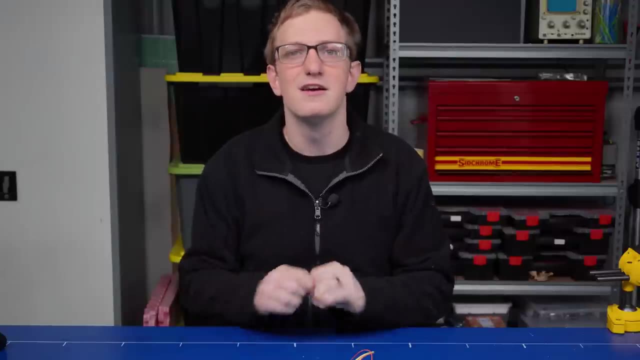 you might choose to implement a motor controller and a robot controller on one processor to eliminate the need for a driver, Or you might be using different types of motors, like steppers or brushless, that work a little bit differently. Regardless, it's probably going to fit this. 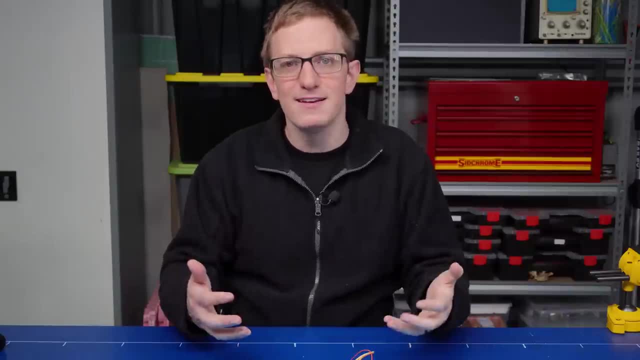 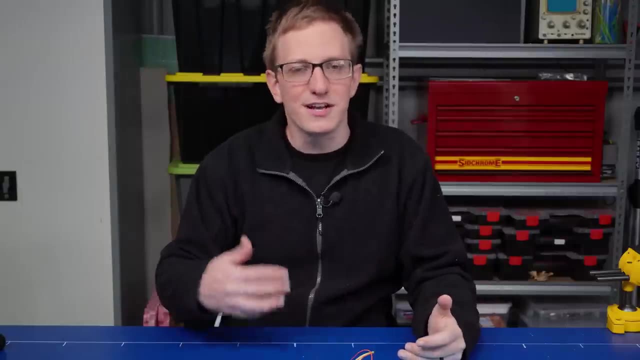 structure in some way. Having a diagram like this is great, but we're going to learn a lot more by getting stuck in and building one for ourselves. So I'm about to make a demo circuit and I encourage you to go out, get the parts and do it for yourself at home. 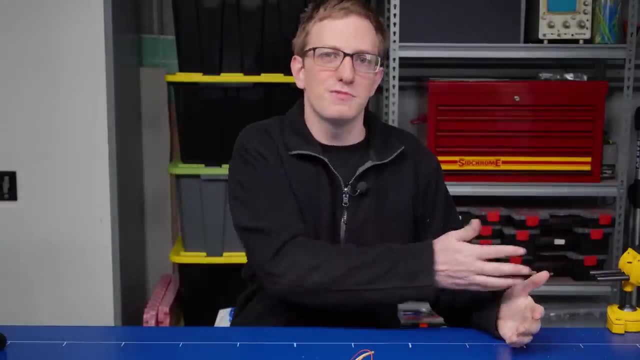 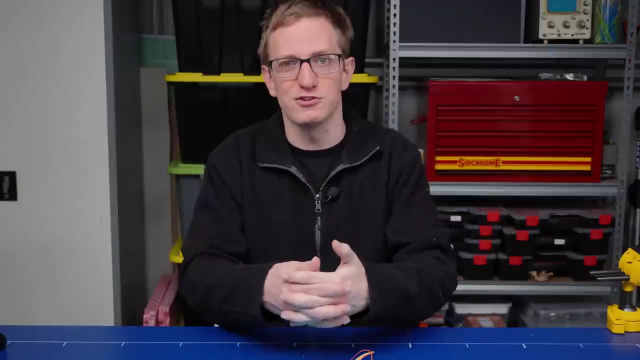 This video is actually part of a larger series where I'm going through how to build an autonomous robot from start to finish. Make sure you subscribe if you want more of that, But for that project I'm eventually going to be using ROS2 control. I'll be using the DiffDrive. 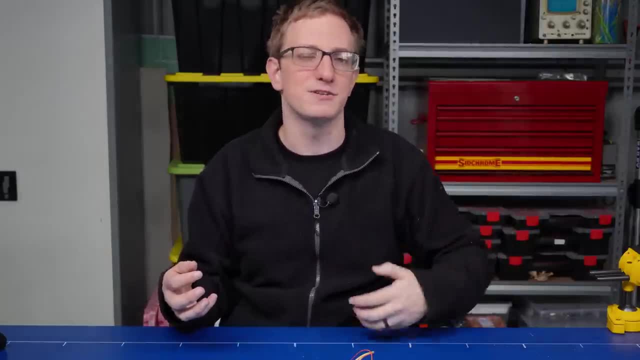 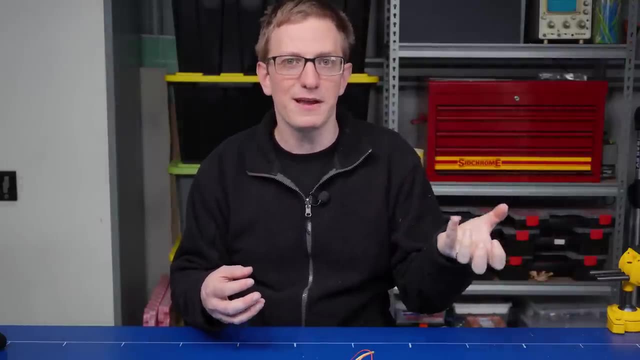 controller that it comes with, and I've written my own hardware interface, which I'll make available on GitHub For this video, though, I've just written a simple driver that uses regular ROS, So it's listening for speeds on a topic, and then there's a graphical interface that you can 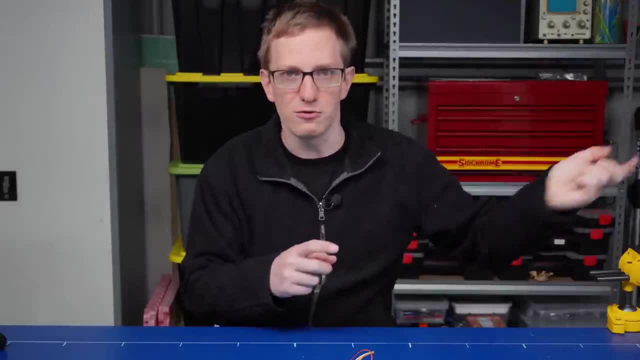 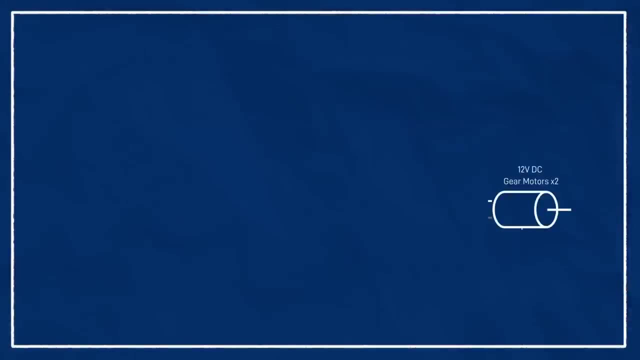 use to request speeds. it'll send them via serial and then it'll report the information back to the graphical interface. Here's a quick overview of the circuit I'm going to be building. I've got two motors- although we'll start by wiring up just one of them- And they're connected to an L298N. 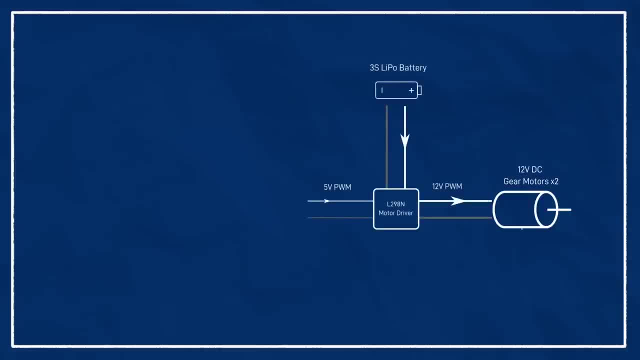 motor driver, which is getting its power from a 3-cell LiPo battery. That is then connected to an Arduino Nano. that's acting as our motor controller, And we've got it also connected to the encoders of the motors so that we can get speed feedback. 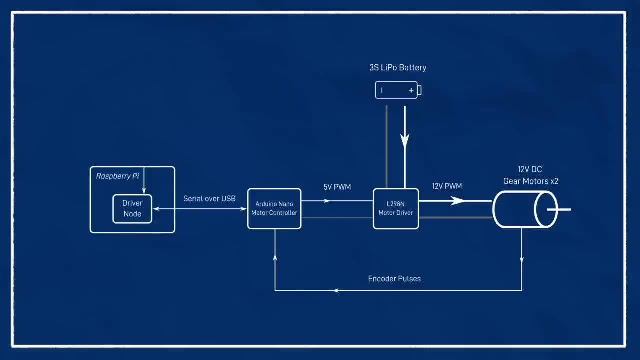 for closed loop control. Then I've got a Raspberry Pi running a driver node in ROS, and it'll be communicating over serial, over USB, to the motor controller, giving it the speeds. And then, instead of having the robot controller on board, like we would have in a real robot for this demonstration- 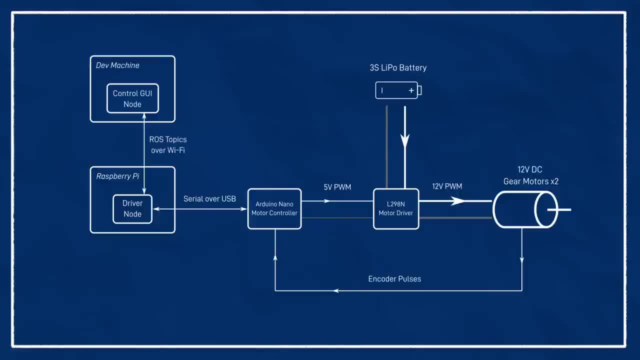 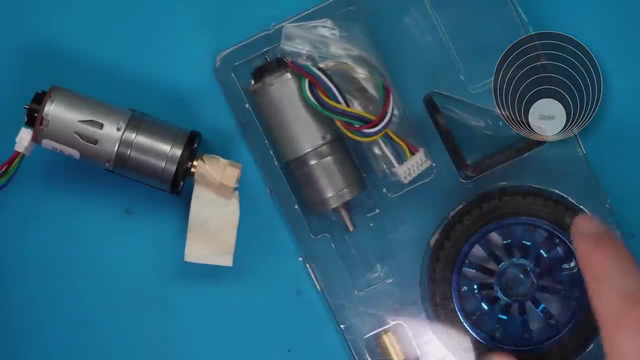 I've just got another ROS node that's going to run on my dev machine and it'll pop up with a little graphical interface that we can control the motors with And it'll be sending the data over ROS2.. So here's my motor. It's a 12-volt DC gear motor and it came with a mounting bracket. 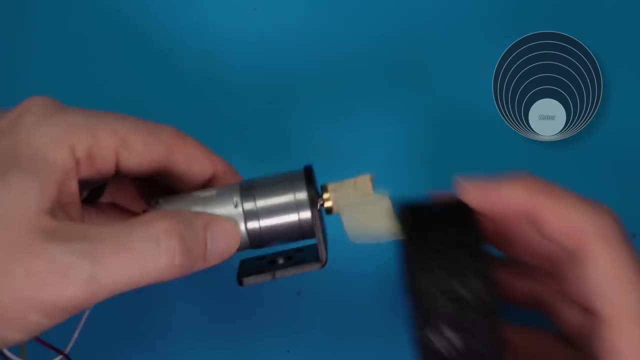 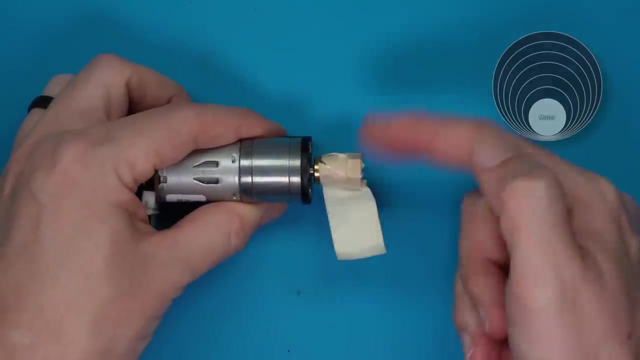 and a wheel, But I'm not going to put the wheel on just yet, because it's taller than the mounting bracket, and so then I'd need a way to prop it up to stop it from spinning away on the table. Instead, I've just stuck a piece of tape around the shaft. That way, 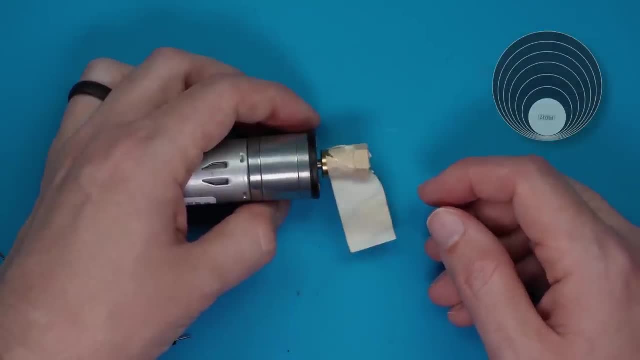 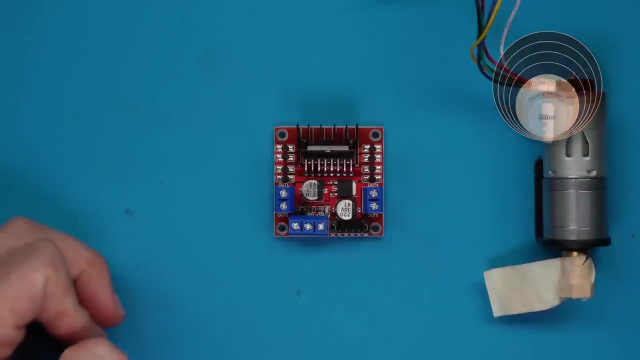 it won't catch on the bench, and it also makes it easier to see how fast the motor's spinning. Next up is the motor driver For my robot. for this example, I'll be using the popular L298N driver. Now, honestly, this is not a good motor driver. It has a maximum of 2 amps of current per. 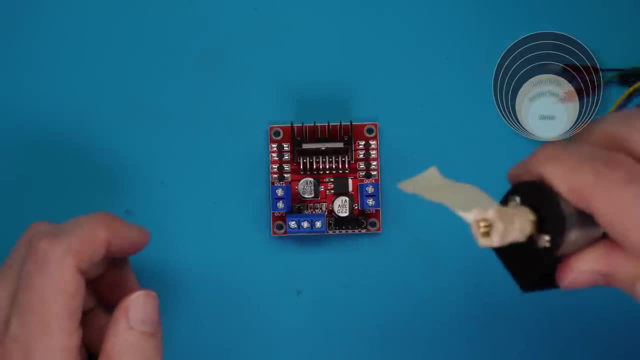 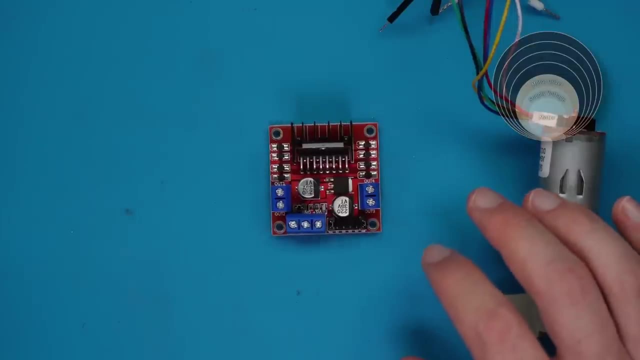 motor with 3 amp spikes, and that's fine for these motors that have a 1.8 amp stall current, but you wouldn't want to be driving something much bigger. Also, it's got a pretty decent voltage drop. So, even though we'll be putting in maybe 11 to 12 volts from our battery, 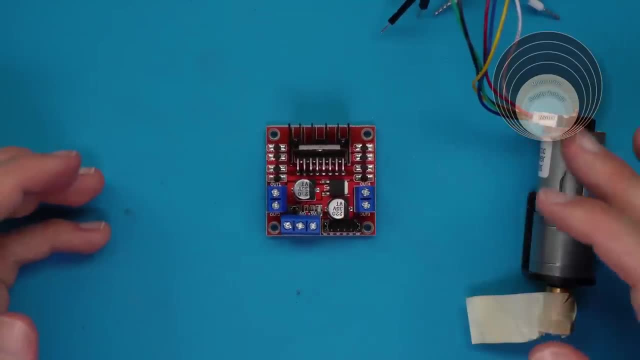 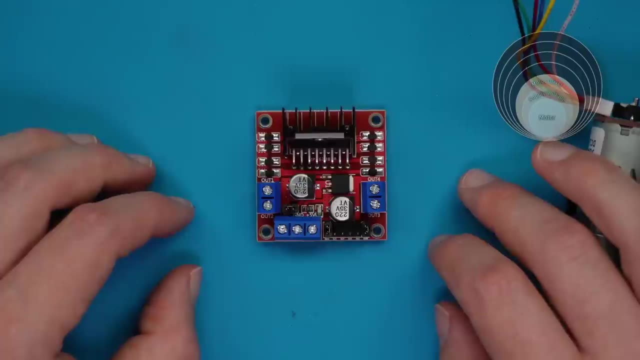 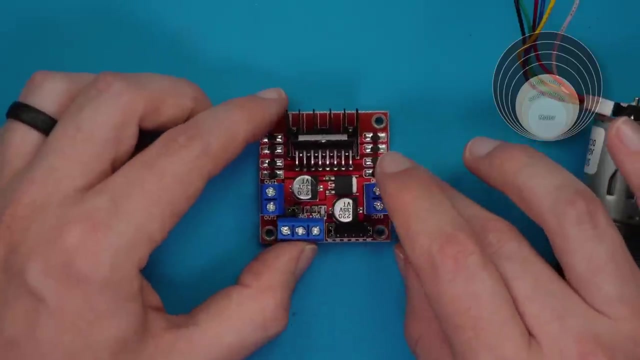 it's only going to be getting 9 to 10 volts out, So our motor's going to be running at like maximum three-quarters speed. Let's take a closer look. Something useful to understand is that L298N refers to the actual chip that's doing all the hard work, and this is just a popular board that this 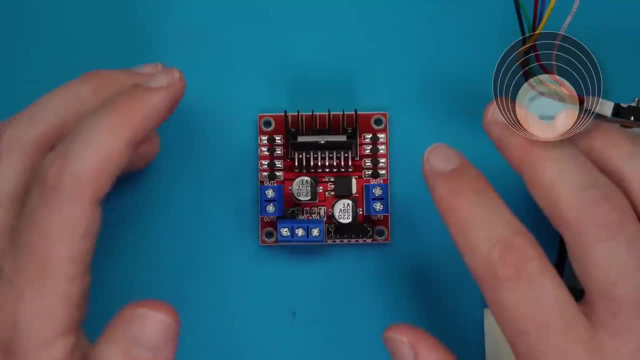 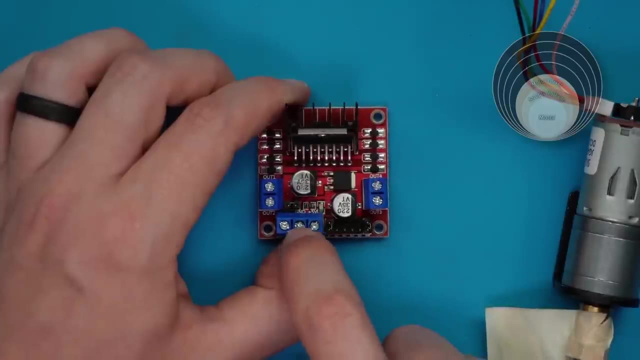 chip comes on that has some extra terminals and stuff to make it easier to use. So we've got 12 volts in to power our motors, We've got 5 volts in to power the chip itself and a common ground. Then we've got a pair of terminals on each side and these will supply. 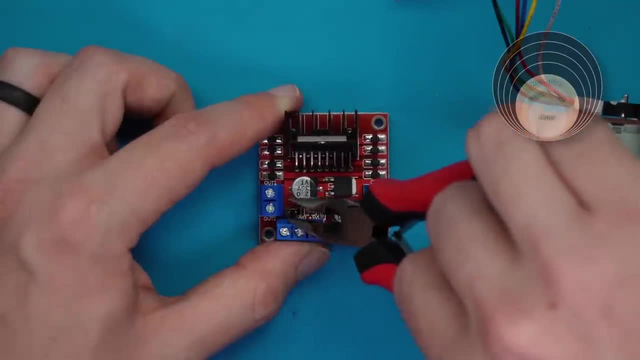 power to our motors. This little jumper here enables an on-board power supply. So we've got a power supply here. This is the power supply. So we've got a power supply here. And then we've got a on-board 5-volt regulator, which I'm going to remove because I've got my own 5-volt power. 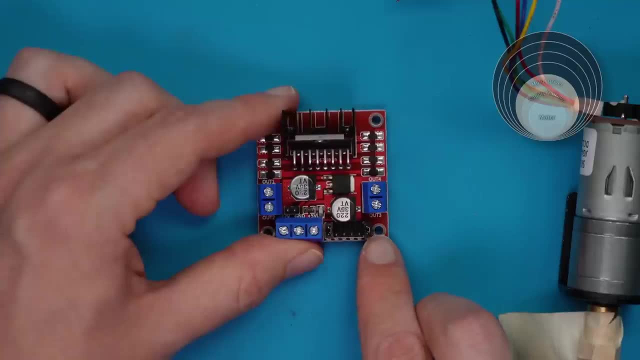 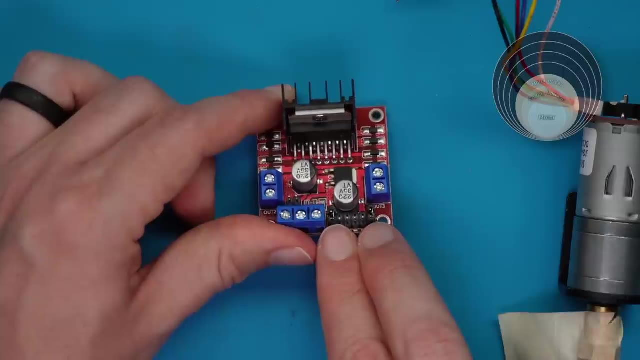 supply, and I don't want them to conflict with each other. This row of six pins here at the front is what we use to control the motors. Now, normally, you'd use the two outside ones to control the speed of each motor, and then the other. 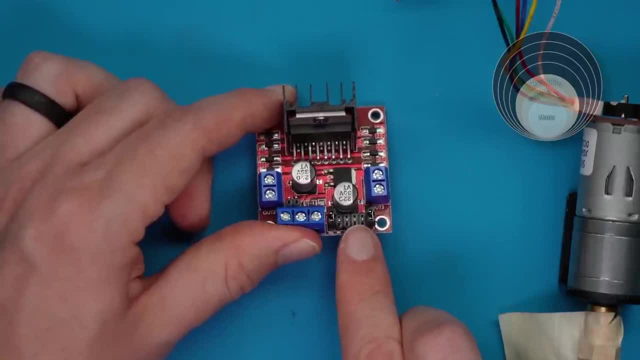 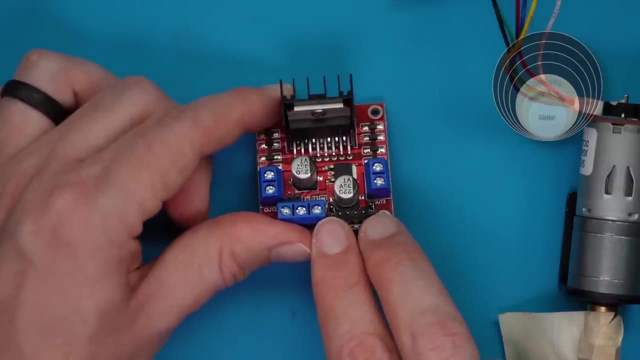 two pairs are used to control the direction, And so when you want to control the speed, you need to remove these two jumpers, because they're currently tying those pins to 5 volts, forcing the motor to go at full speed. However, the controller that I'm using actually expects. 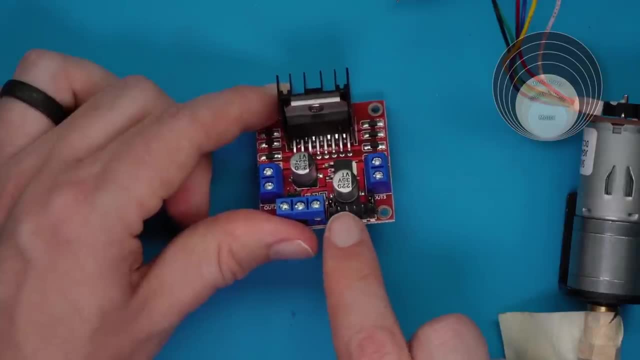 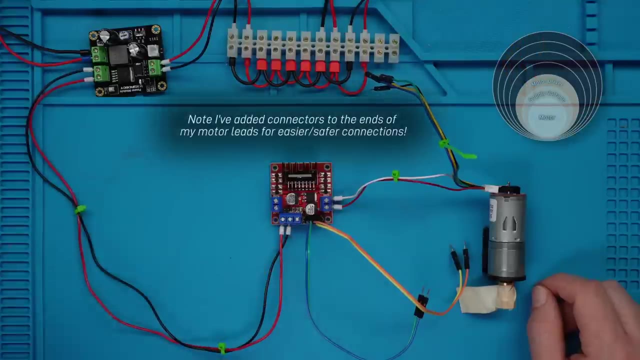 these jumpers to be left on and it uses the other four pins to control both speed and direction, So I'll be leaving them there. So I've connected up the 12-volt to the pass-through voltage of our regulator. You can check out. 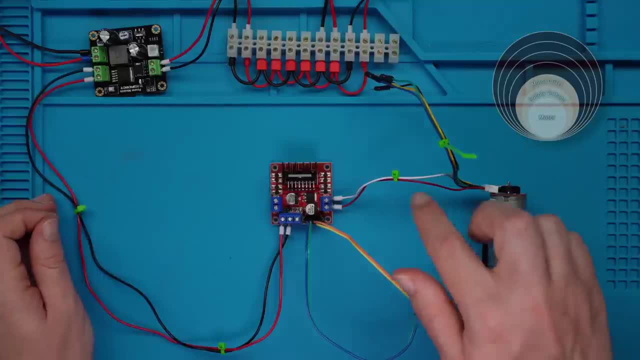 the last video for more information on that. I've got the motor's power leads connected to the output terminals for motor 2.. If you get them the wrong way around, it just means that your motor's going to spin the other direction, so you don't need to worry too. 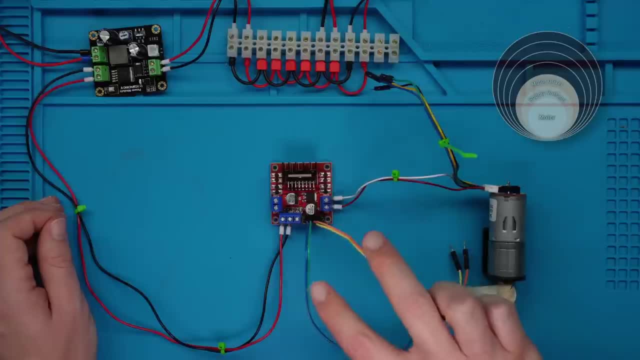 much about the direction of them just yet. Then I've got two pairs of jumper wires coming out of the motor control pins, And then, finally, I've left the 5-volt terminal empty, and we'll see why in just a minute. 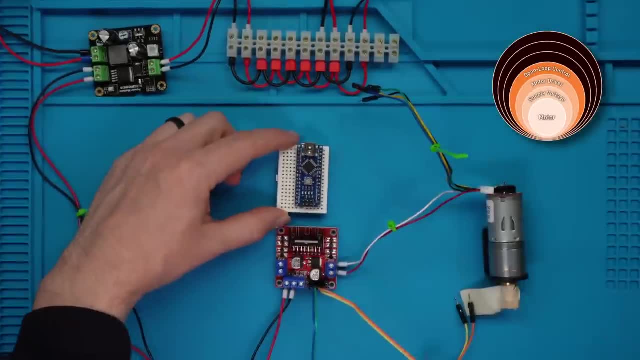 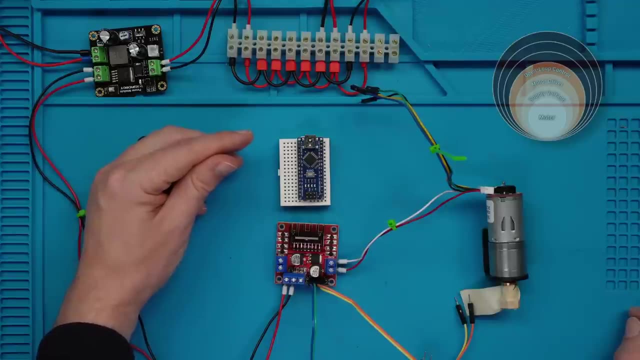 For the motor controller, I'll be using an Arduino, specifically an Arduino Nano clone. You could also use an Arduino Uno. I'd like to redo the controller from scratch one day, maybe with a different chip like the Raspberry Pi Pico, but the Arduino works totally fine. 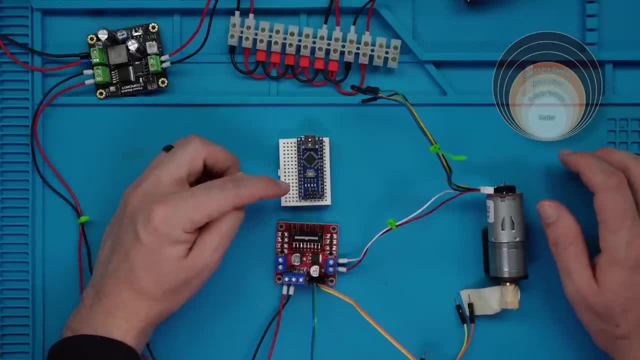 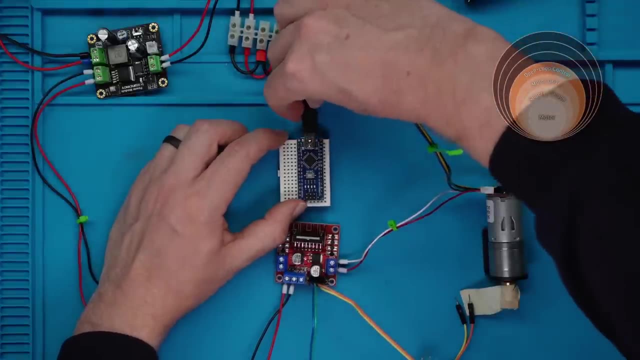 for now. I had planned to power the Arduino using the 5-volt pin and only use the USB for serial problems, but instead I've decided to let it be powered over USB as well. However, if you remember from the last video, I'm actually going to be connecting it to this powered 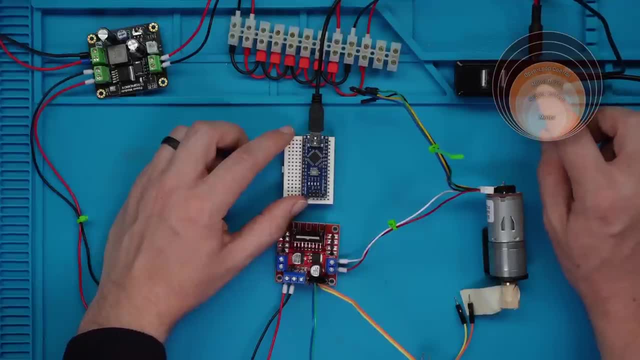 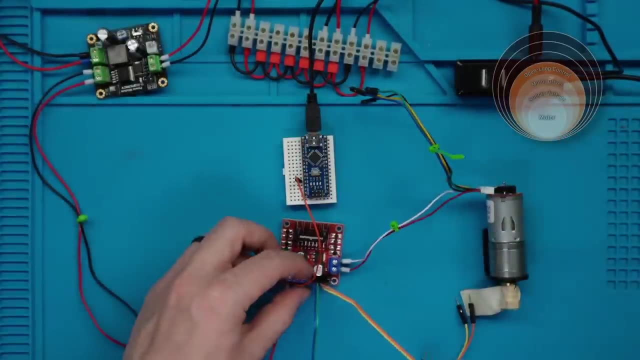 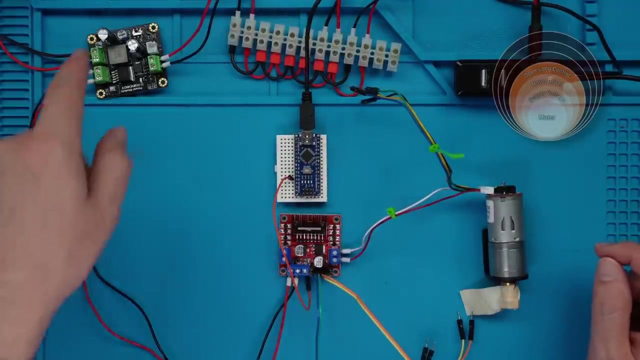 USB hub and that way I'm going to minimise the amount of current that's being drawn from the Raspberry Pi. Then we can piggyback the 5 volts from the Arduino into the motor driver And the ground is shared through the whole system back via the regulator. 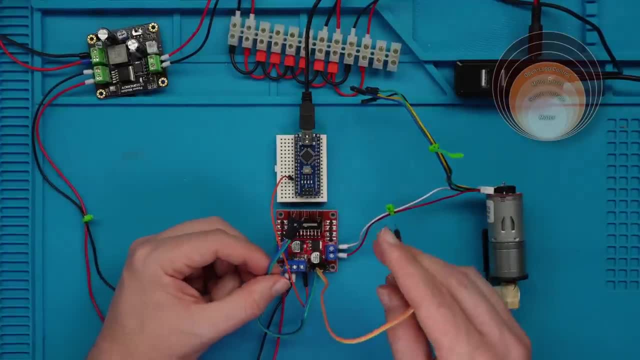 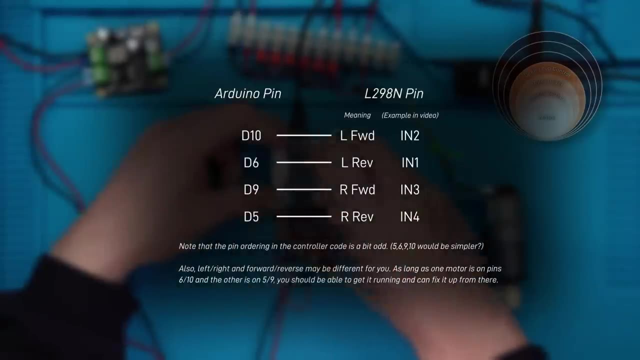 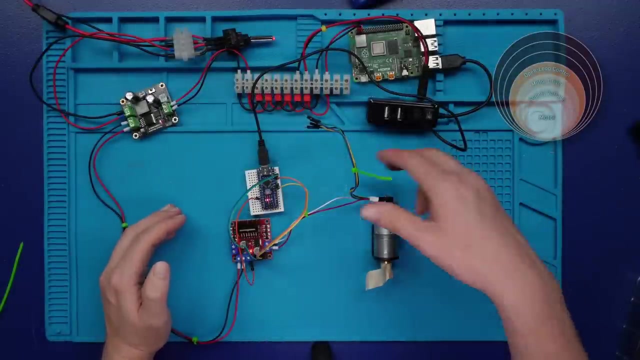 Then you want to run those other 4 wires from the driver pins to the Arduino pins according to the diagram, Although I'd probably wait until you've uploaded the code first before you go ahead and plug it all in. We've got the hardware for our motor controller mostly done, apart from these 4 wires which 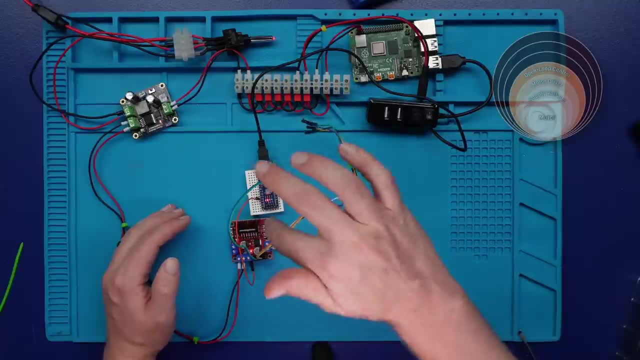 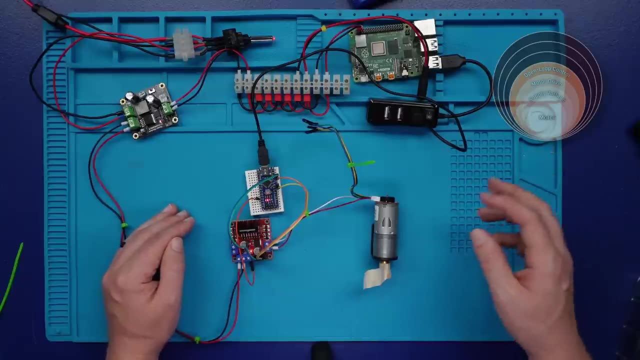 are for our encoder. We'll set that up soon, But first we're going to upload the code to the Arduino. I'll be using a modified version of some code that I found online. Now, I didn't write this code. I can rewrite it from scratch one day, But in the meantime, thanks heaps to the original. 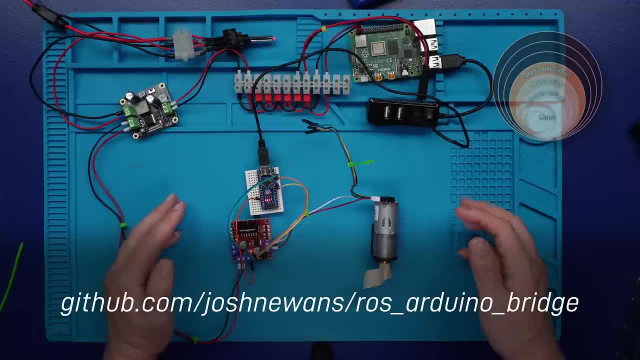 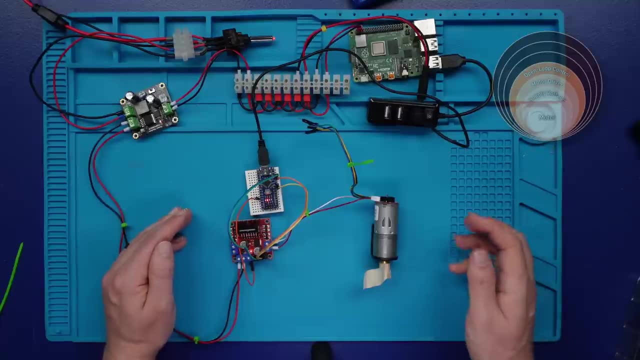 authors for creating it. You can download the code from my GitHub and upload it using whatever method you like. I just made a video on a couple of different ways to do it and the way that I think is best, So you can go check that out. I'll include a link in the description. 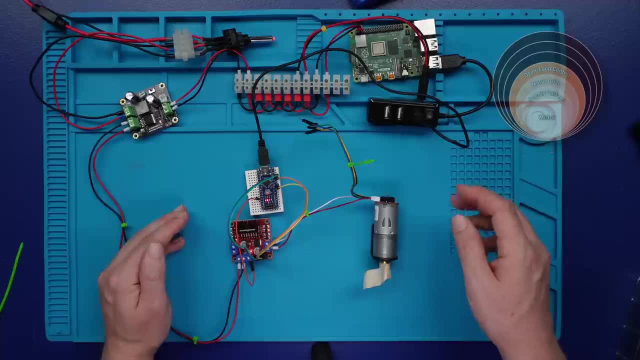 And unless your hardware is exactly the same as what I'm using, then I recommend you read the README file first, just to check if you need to make any changes before you upload the code. Once the code is uploaded, we can test if our serial comms works. I'll be using a 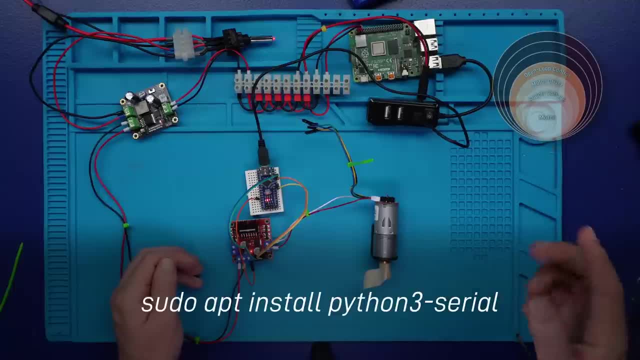 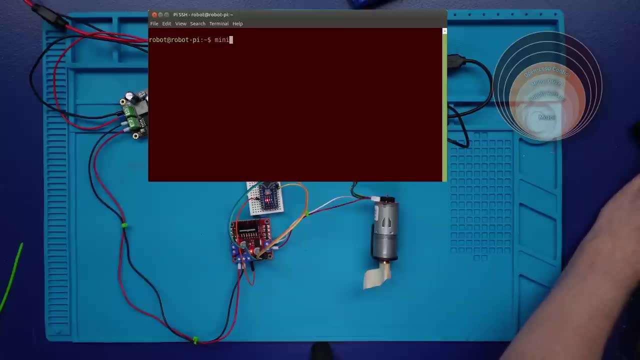 program called Miniterm, and you can install that using the command up on the screen. if you don't already have it, Assuming you've got serial access enabled on your Pi, then you can type miniterm-e for local echo, then the serial port, so for me, sadd slash, dev slash, tty, usb 0, and then the. 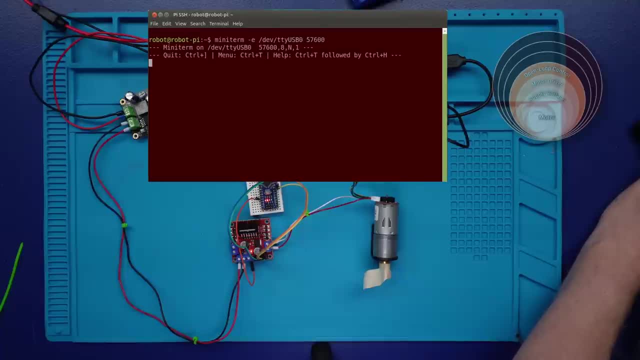 board rate, so 57600.. And so I can type e to check the current encoder values. They're 0 because we haven't plugged them in. But then what I can do to check things are working so far, I can type 0,, 255,, 255. And this tells it to run both motors at full speed in open loop. 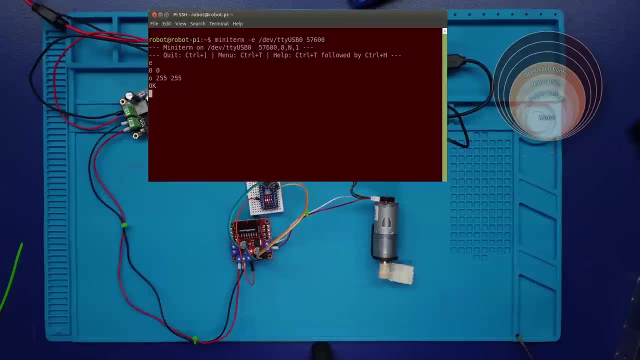 raw PWM mode. Sure enough, the motor spins around, Type 0 and 0 to stop it Now, because I've only got motor 2 plugged in, I should be able to type 0,, 0,, 70, and run just this motor at a slower speed. 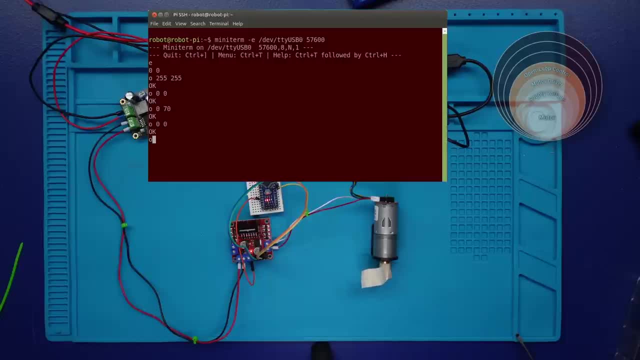 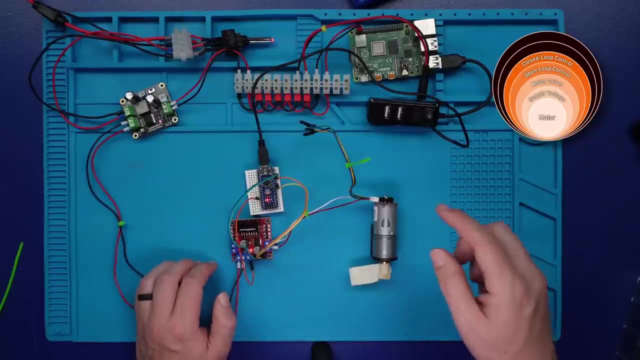 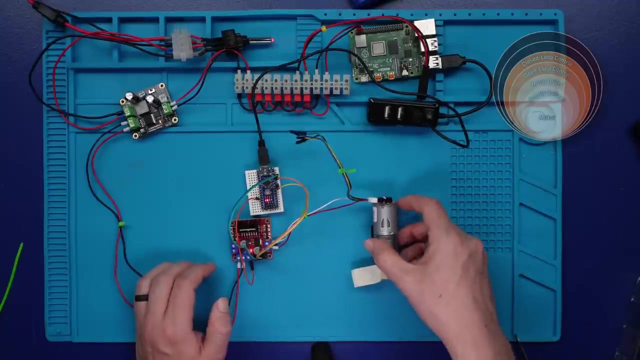 Gloss, And then I can also underside TO to check that that works. So let's go minus 150. And sure enough, it spins backwards. Now that open loop control is working, we want to implement closed loop control And remember from earlier. that means we need speed feedback back from our motors to the 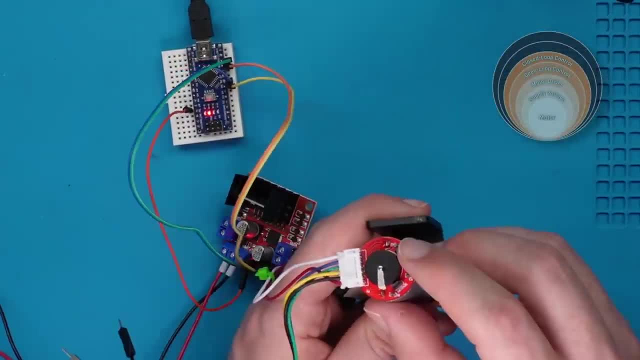 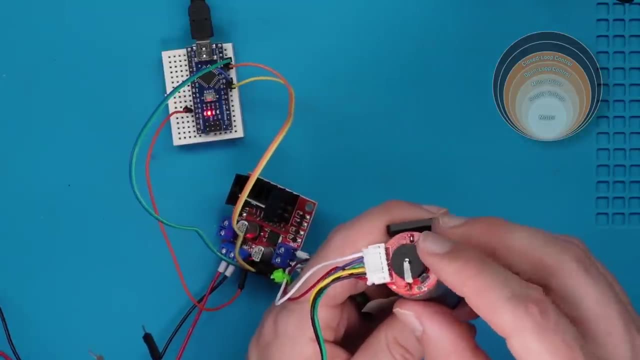 controller. We can solve this problem using encoders On the back of this motor. here you can see On your motor. they might be covered up or there might not be one at all, in which case you can buy them to install Yourself. but I recommend getting them pre-installed and then, as the motor spins, 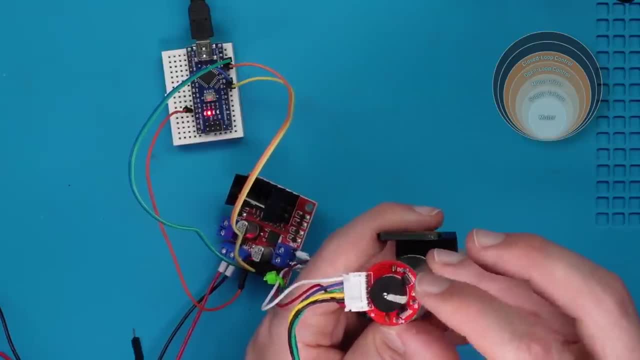 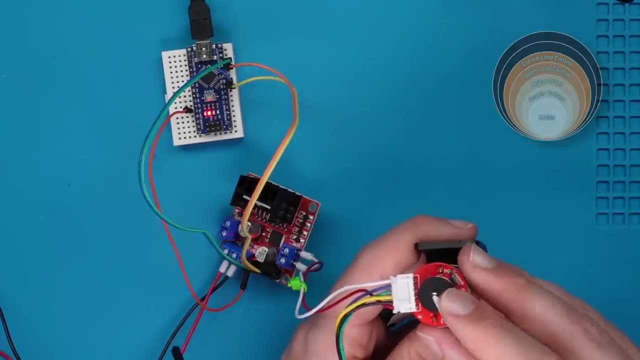 The magnetic field of the disc is gonna go past these little Hall effect sensors And they'll send a signal that goes up and down in pulses back to the controller. I've put a bit of tape on mine so that you can see the spinning easier. Usually they'll just be all black, and so for each revolution of this disc. 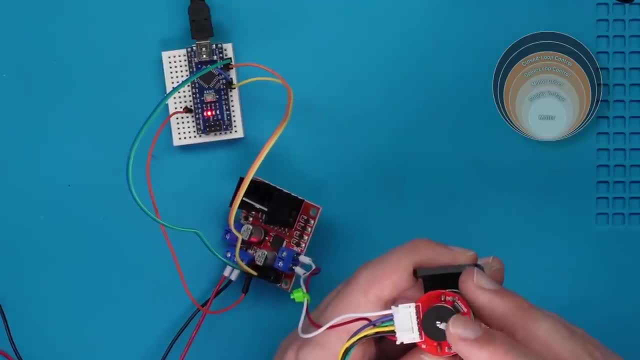 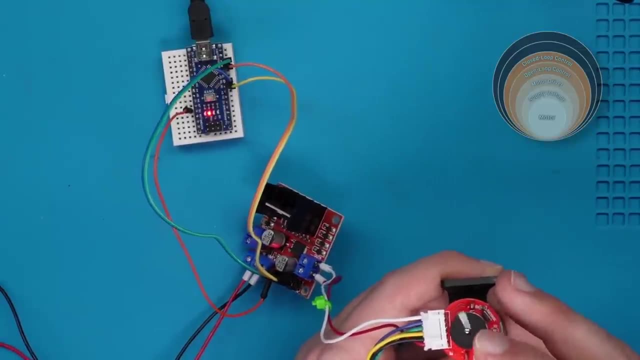 You're gonna get the signal go up and down a certain number of times, not heaps of times, Maybe like eight times per revolution for a cheap one, Maybe even over a hundred on a good one, and that might not seem like a whole lot. But you've got to remember that this is going through a gearbox. 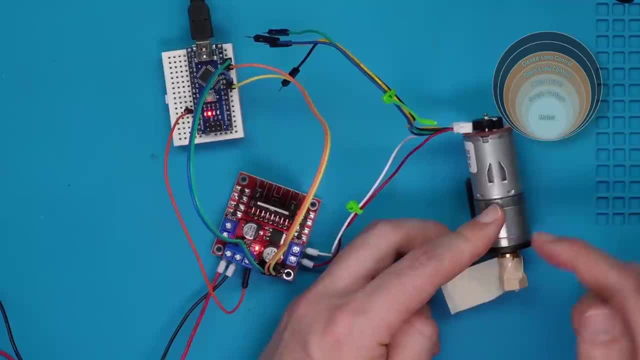 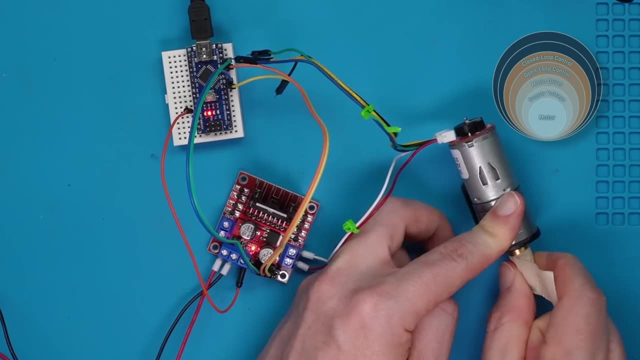 And so each revolution here is going to be only a fraction of a revolution on this side, And so for one revolution on this end, you might be getting like a hundred turns on the other end. So if I spin this, you can see that spinning many, many. 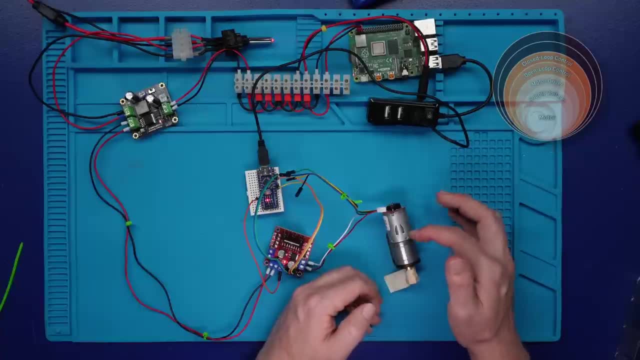 times. As to how the controller is able to convert these blips into a measured speed, We're not going to go into too much detail. If you want a video on how encoders work, let us know in the comments. I might make one down the track. 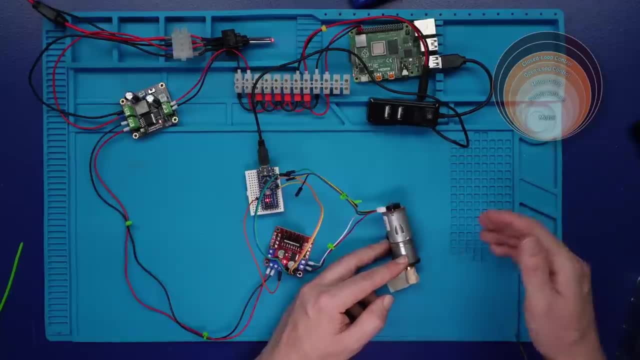 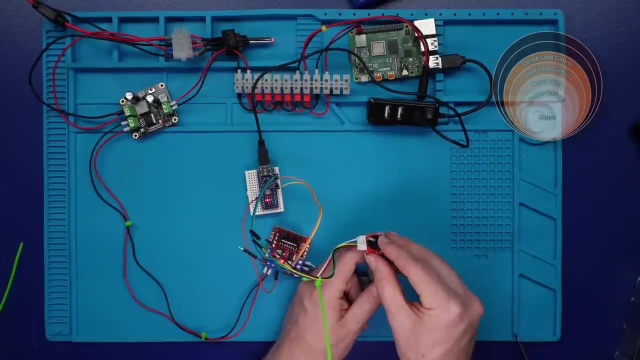 But basically it's able to convert these blips into a count That's going up and down as it turns and then by checking that counter regularly, say 10 times a second, and noting the difference in the counts, We're able to calculate the motor's speed in counts per second. 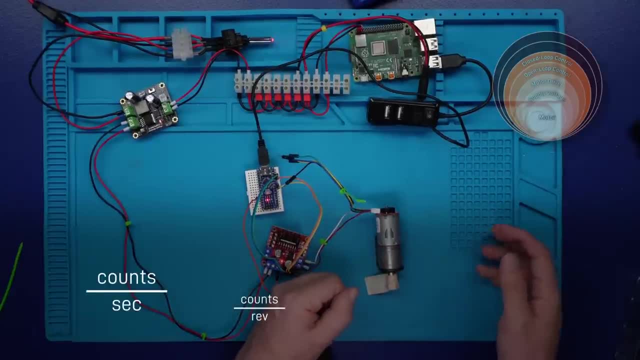 Then if we know how many counts there are in a full revolution, We can convert that counts per second speed into RPM, degrees per second, radians per second, Whatever we like. now for these particular encoders, We've got four wires, two of them are going to go to five volts and ground. 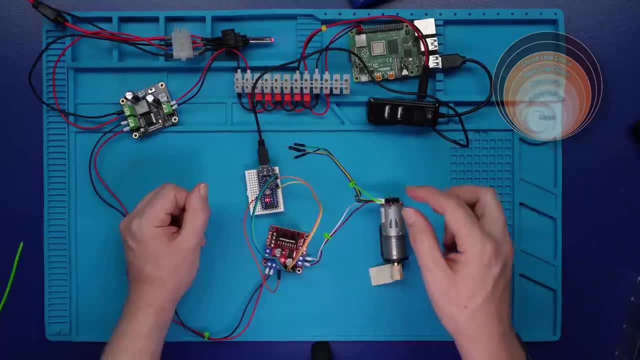 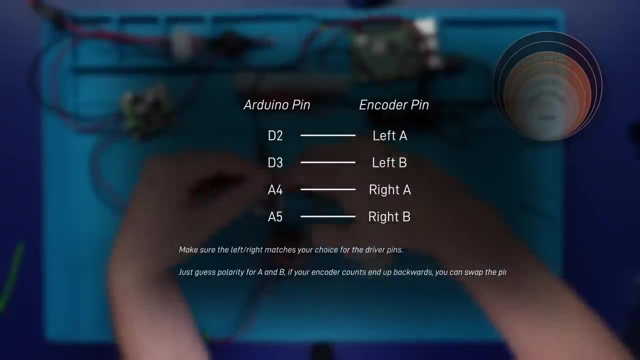 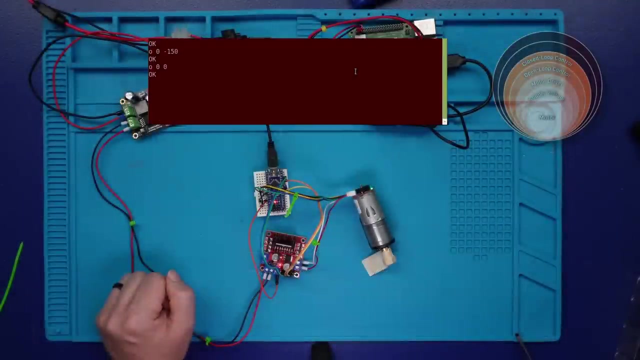 That'll give power to the encoder circuitry, and then the other two are going to go to input pins on the Arduino. I'll put them up on the screen Then, going back to our serial terminal, we can run the E command to read the encoder values now, if they're not already zero. 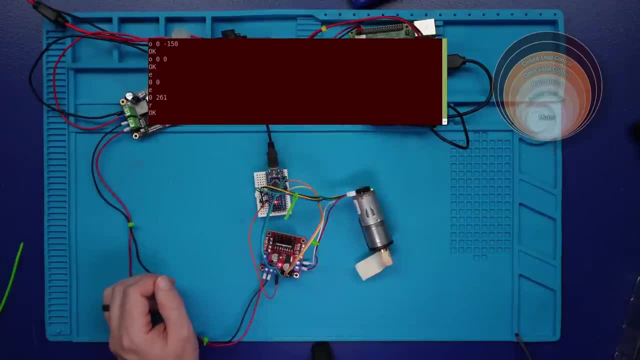 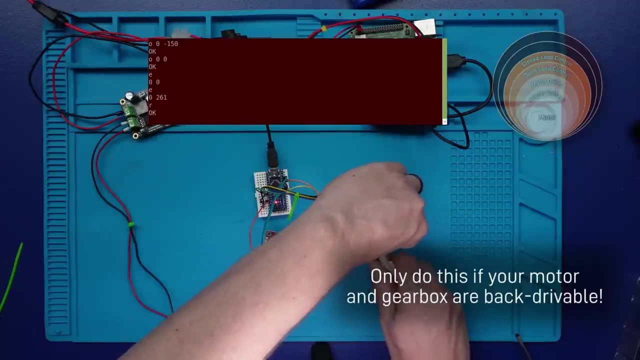 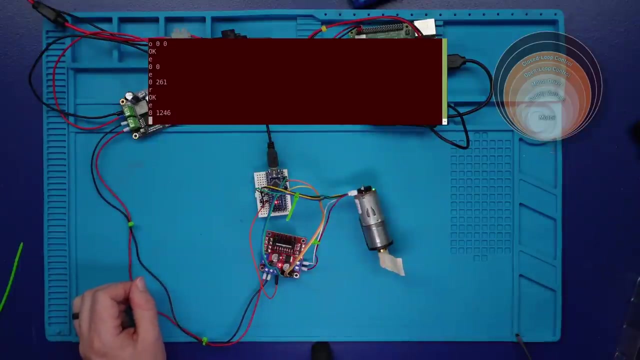 then we can just press R to reset them and Now we can turn the shaft in whatever direction was positive when we were doing open-loop control before. if you haven't got a wheel connected, it can sometimes be a bit hard to turn, and When we hit a we should see a positive number in the reading. if it isn't, then we just want to swap the the two. 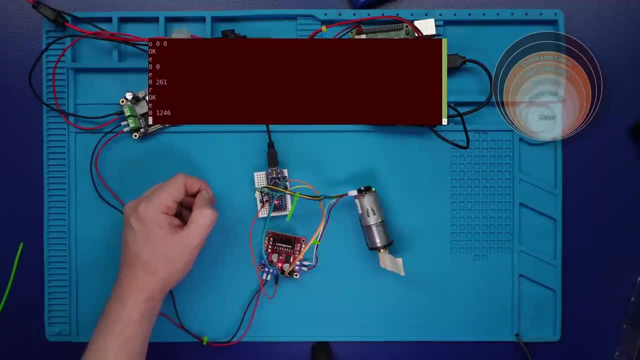 Wires that are going to the Arduino, reset With the R command and try again Now to control it properly. we're going to need to know our total counts per revolution of the output shaft. We could figure this out by looking at the data sheet and multiplying the encoder counts per revolution by the gear ratio. 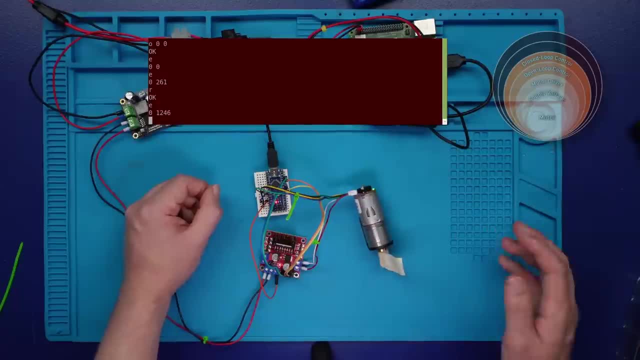 But I don't always trust the data sheets, and for cheap motors like this you might not even have one. The best way to do it is to just measure it ourselves empirically. So we'll hit R again to reset the measurement, and then we want to rotate the shaft a whole lot of times maybe. 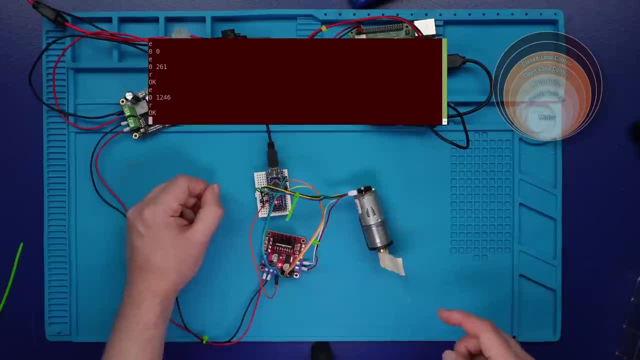 10, 20, 30 times, and then we'll divide what the final count is by The number of times we rotated it to get the counts per revolution. So we'll check the encoders. There's zero. I'm going to cheat by just running it in open-loop control for a while. 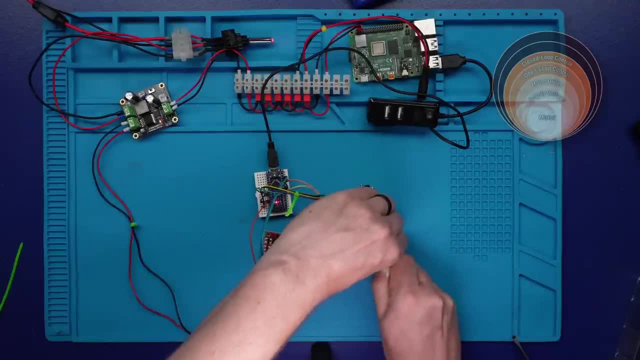 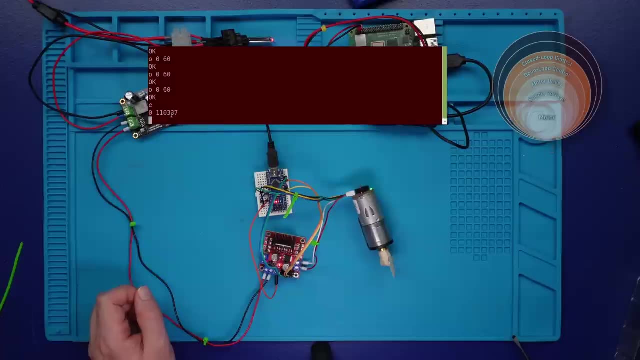 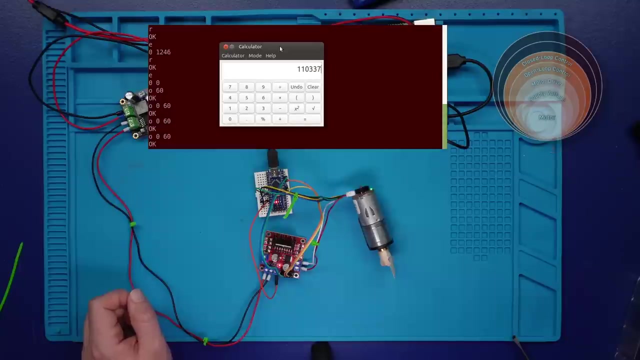 And then I'll just finish this one up, Try to get it back to where I started. I think it was about there. So we'll check the encoders and we're reading 110,337. So I'll open up the calculator- 110,337 divided by 32 revolutions, and we get. 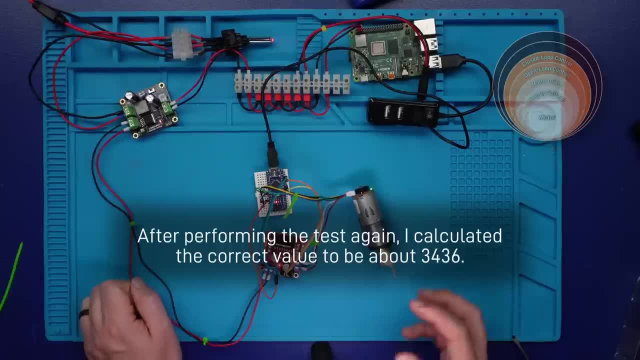 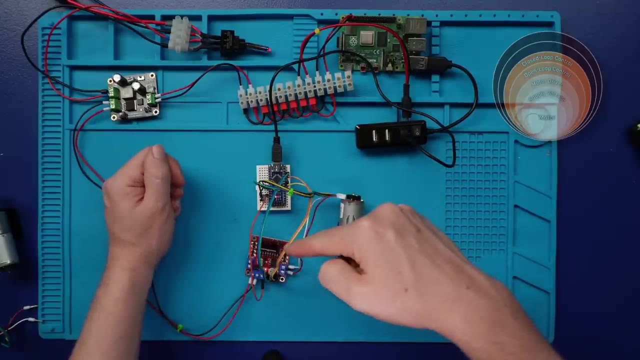 3448. So that means for each revolution of the output shaft we're getting 3448 counts. I'll round that up to 3450, And so that means we can calculate the actual speed that it's going, Now that we can send a control signal to our motor driver and receive speed feedback from the motor. 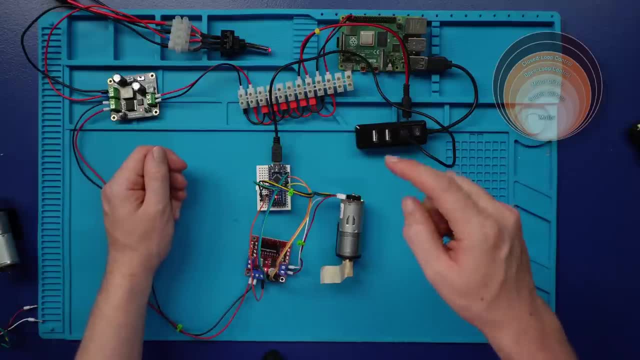 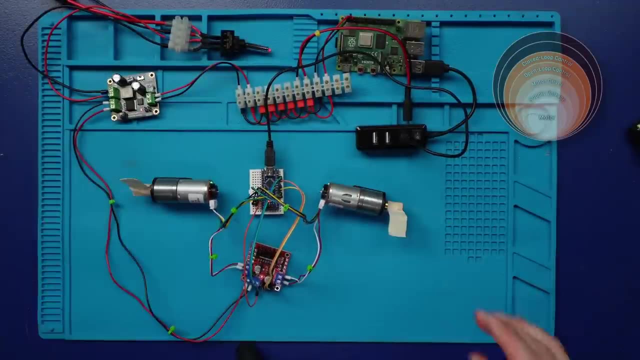 That means we're ready for closed-loop control. But before we do that, I'm just going to get a second motor wired up. Now, the way that we tell this particular controller how to go is with number of encoder counts per PID loop. is with number of encoder counts per PID loop. 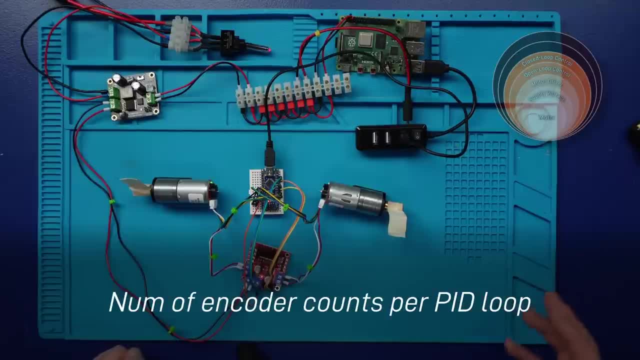 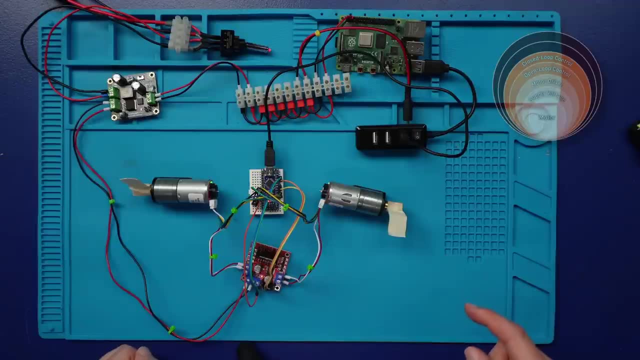 It's a bit of a weird unit. I'm not a huge fan of it, but we'll just roll with it. Now, the PID loop is set to run at 30 times per second, So if we want to make motor one go at one revolution per second. that's going to be. 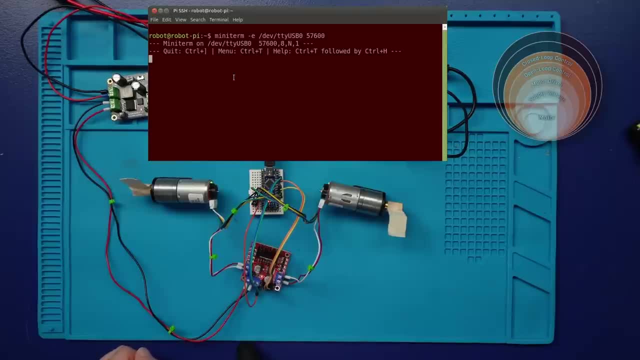 115 counts per loop. So I'm just going to check that open-loop control is still working, And now let's try a closed-loop control. So for that we use the M command. So I'm going to type M 115, 115, and we should see each motor turning at one revolution per second. 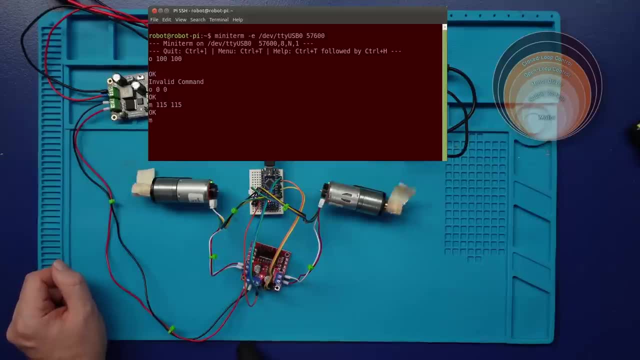 And we can try backwards as well. Let's go maybe half that Now. for my motors the default PID parameters are fine. If you do need something different, you can tune those parameters. if you check out the readme in the code repo, It explains how to do that. 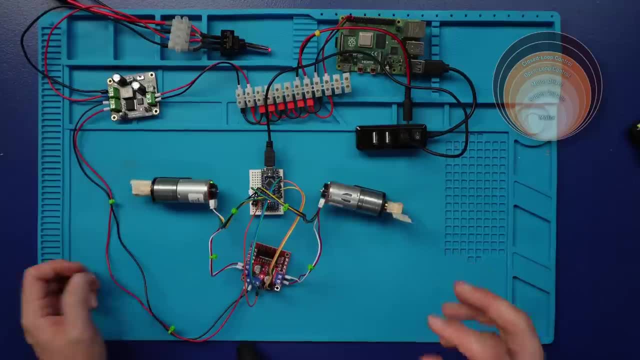 So now that closed loop control is working, we want a way that we can interact with it from our higher level. For a simple robot, you could do it all on an Arduino, but for anything more advanced, you're going to want something with more grunt. So for my 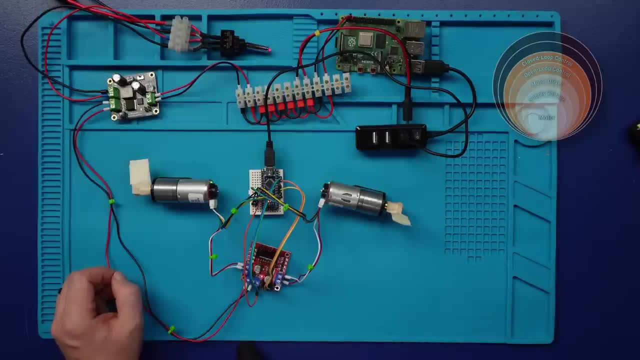 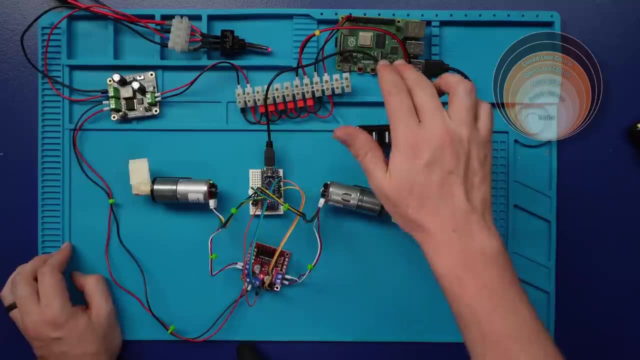 robot. I've got a Raspberry Pi on board connected to the Arduino, So I've got a little demo that we're going to run. It comes with two ROS nodes. One of them is going to run on the Raspberry Pi and that'll be listening for motor speeds on. 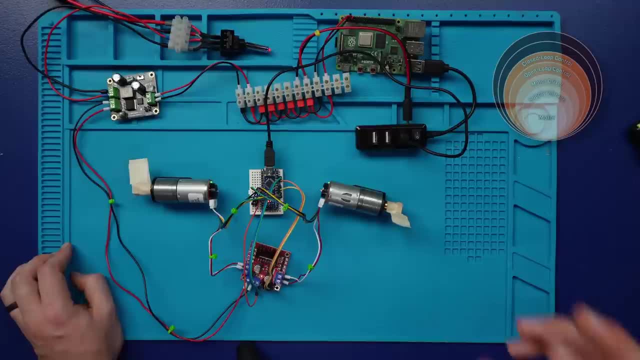 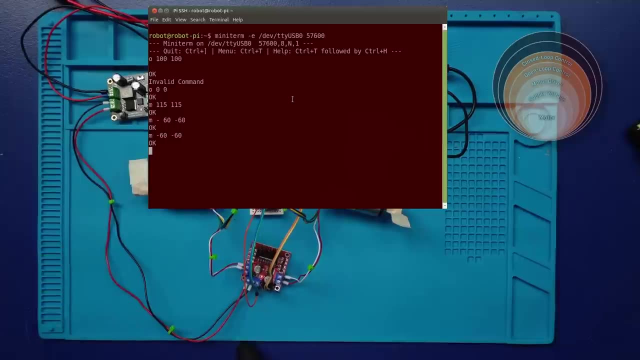 a topic and sending them to the controller. And then there'll be another node that's a GUI that'll run on my development machine where I can send commands in a more user-friendly interface. So I'm going to clone that repo into my workspace. 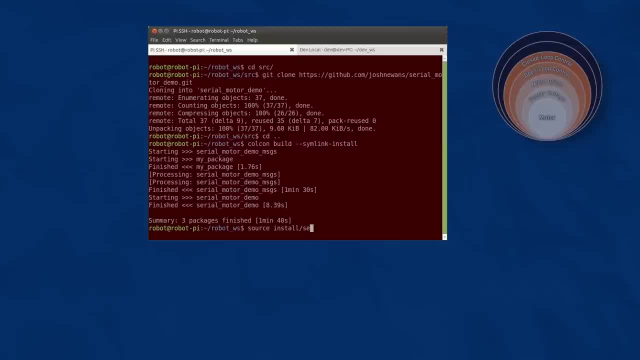 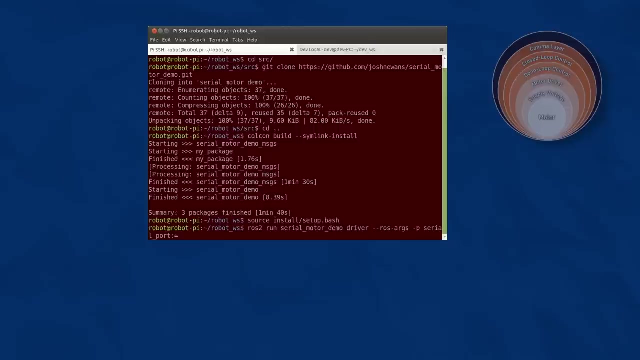 Now we can source our workspace. So on the Pi we want to run the driver, So we'll type ROS2 run. The package is serial motor demo and the node is driver. Now there are a few parameters. we have to pass this, So we'll type ROS args. We've got the serial port, which is slash dev slash. 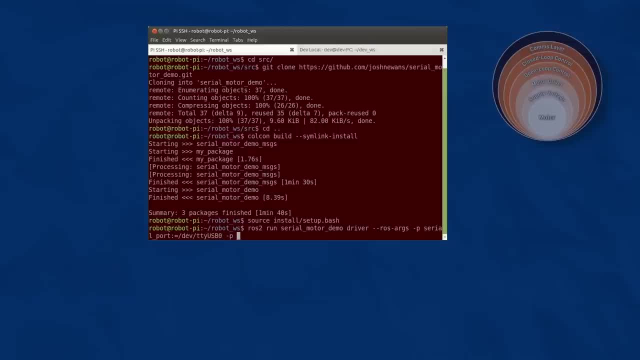 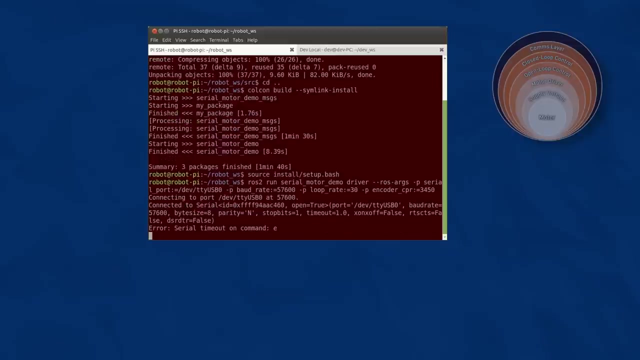 TTY USB 0.. The board rate is 57,600.. The loop rate is 30.. And the encoder counts per revolution, if I remember, is 3450.. That error is okay. So that driver is now listening on a topic, waiting for me to send it somewhere else. So I'm going to. 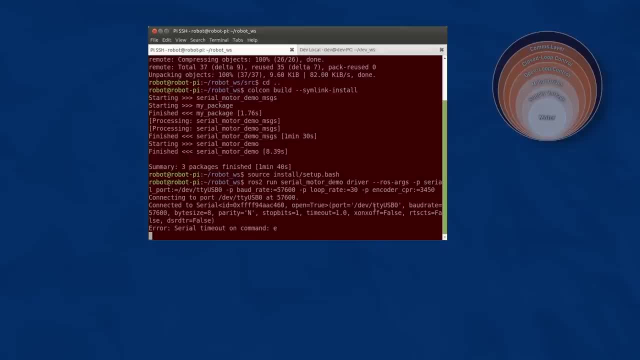 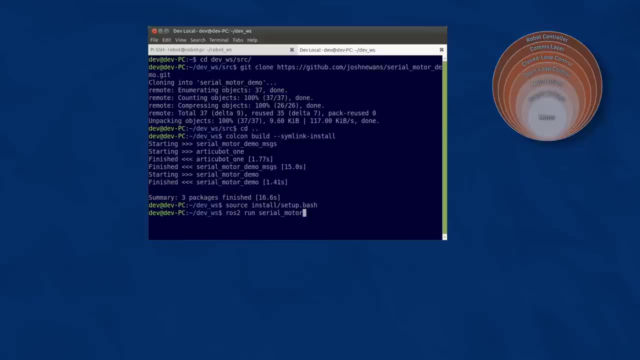 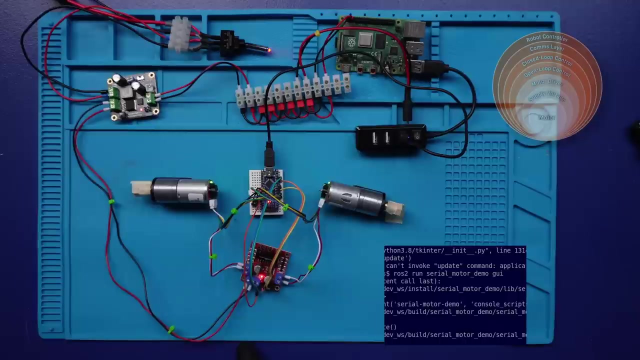 add some motor speeds, which it'll then send down to the controller. So we can now swap over to our dev machine and we can type ROS2: run serial motor demo GUI. There's no parameters for this one, And that'll bring up this little GUI where we 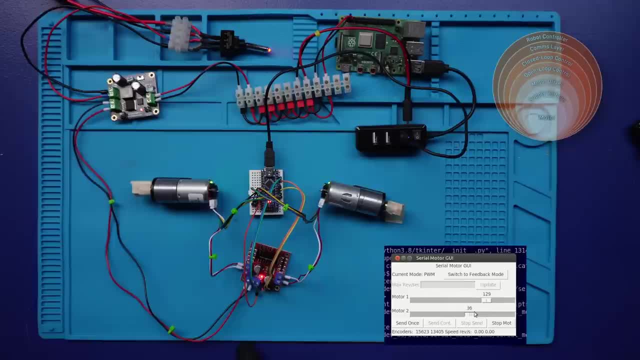 can control the motors. So let's start by setting both motors to PWM, about 130 in positive And yep, that works, So we can stop them. Let's try going negative And they go backwards. We can swap to feedback mode, closed loop control. Now we need to specify the maximum number of revolutions. 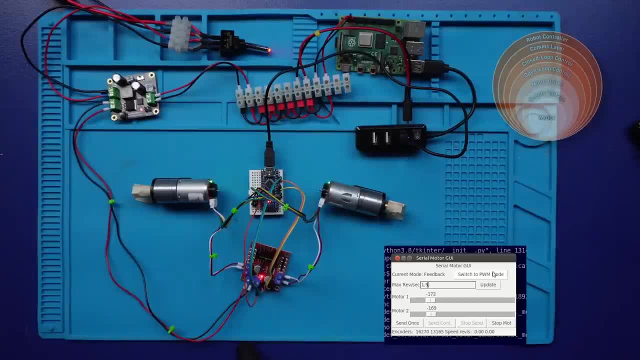 per second And I know that this motor can only do about 1.5.. So we'll click that. It'll update the sliders. Let's set motor 1 to go plus half a revolution per second And motor 2 to go backwards at half a revolution per second, And you'll see. 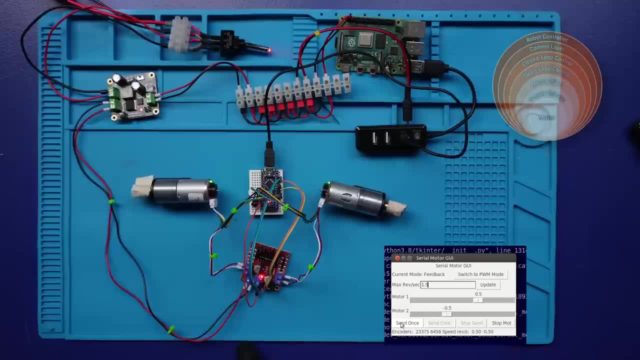 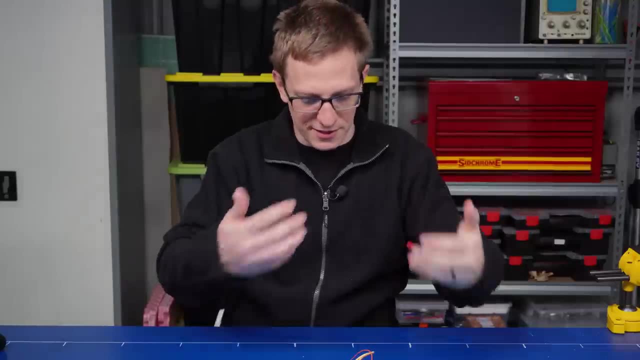 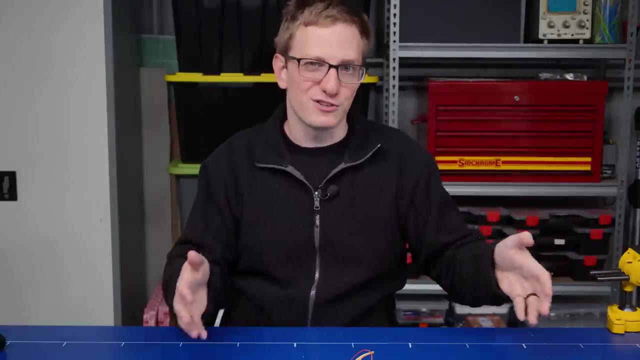 It works, It works, It works. They do exactly that. So now we've got a circuit that lets us control the speed of two DC motors reasonably accurately from a Raspberry Pi and a roadmap on how we're going to be able to integrate that with ROS2 control down the track. 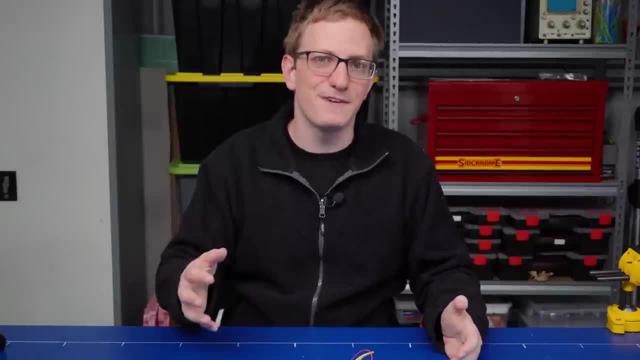 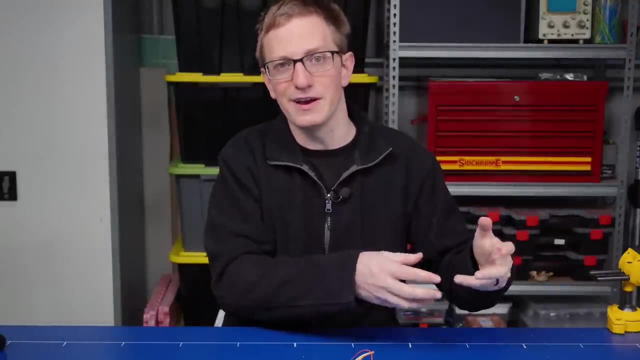 In the meantime, we can start adding some sensors to our robot. So in the next video we'll be looking at LiDAR. We'll go through how LiDAR works with ROS, how to simulate it in Gazebo and then how to integrate the real hardware in our robot. Make sure you. 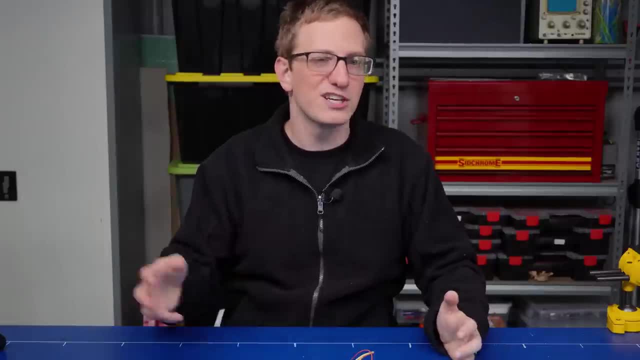 like and subscribe so that you don't miss out on that. If you've got any other questions or comments or ideas, let us know in the comments. Otherwise I'll see you next time.